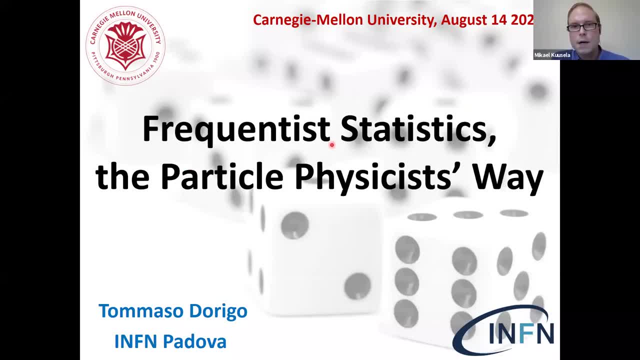 All right, And with that I'll go ahead and introduce Tommaso. So Tommaso is a researcher at INFN in Padova in Italy. He is an experimental particle physicist and he's expertly active in statistics and machine learning in particle physics data analysis. So he has done a long 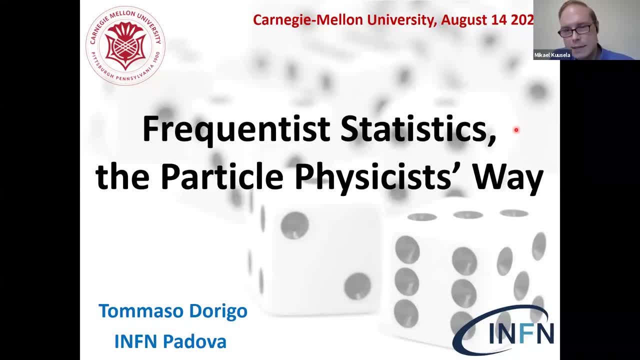 career on that general area, starting with the CDF experiment at Fermilab and more recently with the CMS experiment at the Lodz Hadron Collider at CERN, And he's actually interested in basically statistical techniques and machine learning techniques in particle physics- data. 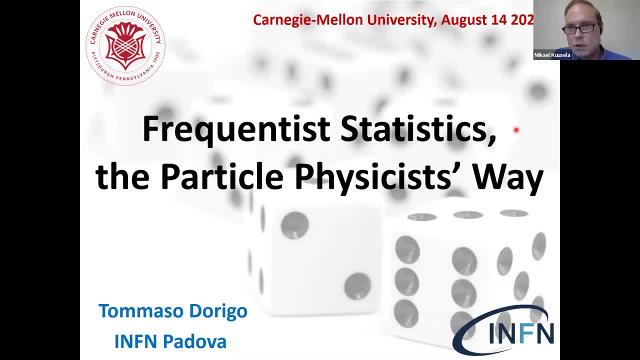 analysis. He has also held various leadership positions in that area. For example, he was for several years the chair of the statistics committee at the CMS experiment, including in 2012 during the discovery of the Higgs boson, So he was effectively overseeing the 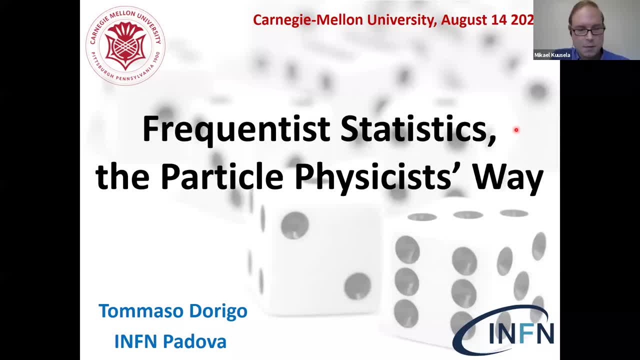 use of statistics in the experiment during that very exciting period of time. After that, he has also managed two separate European training networks on machine learning techniques in particle physics data analysis, effectively training several PhD students in machine learning and advanced statistics in particle physics data analysis, So he's an expert in that area. 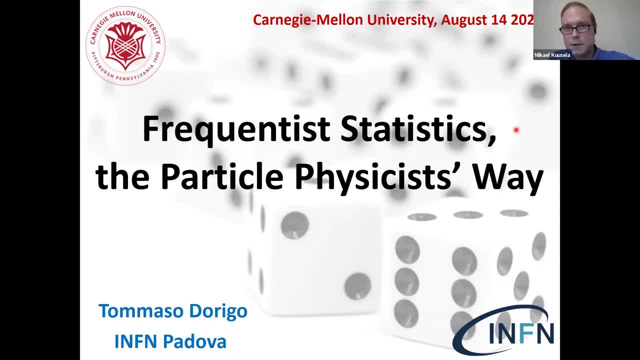 He's also very active in scientific outreach. For example, a couple of years ago he published a book called Anomaly Collider Physics and the Quest of New Phenomena at Fermilab, which I would very much recommend you to read if you're interested in knowing how these large 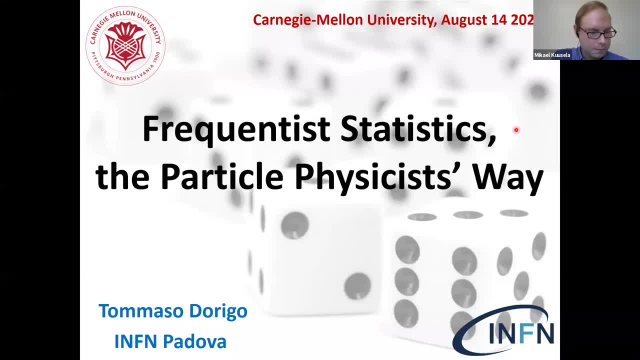 scientific experiments actually function. With that, we will go to the actual talk. So the talk is called Frequent Distance. Okay, thank you, Michael, for this luxurious introduction And thanks everybody for spending your time with me- this evening for me, or this afternoon for you. 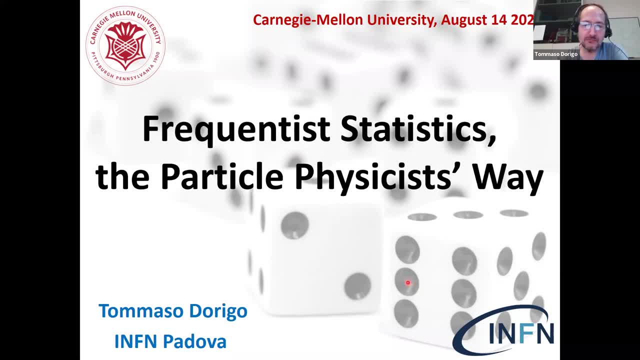 So, yeah, this talk will end here. This talk will try to give you a flavor of the kind of use of statistics that is made in particle physics experiments, And of course we will not be able to cover everything, but we'll give a look at a few interesting things. So the reason for this talk, in fact, as I 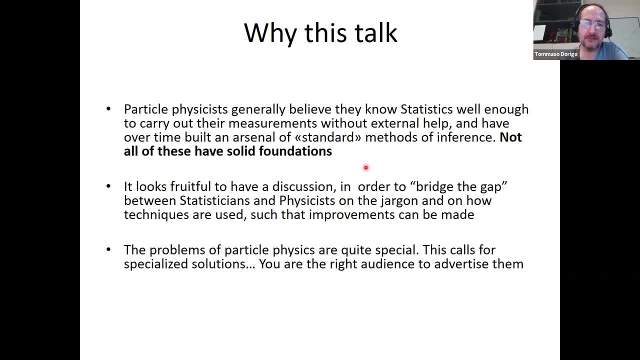 see it is that we particle physicists have the tendency of believing that we can do everything. okay, We can do everything better than anybody else. We are the first in the class, so to speak. That's a general attitude, But in general, physicists think that they know statistics. 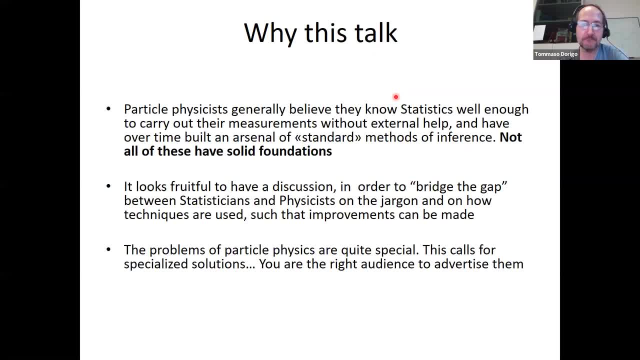 enough to carry out their measurements without external help, And they have, over time, built an arsenal of standard methods of inference, some of which are special to the field, And not all of them, I would say, have a solid theoretical foundation. 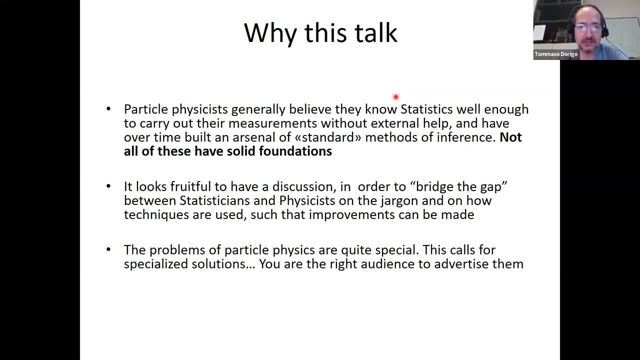 Okay, Okay, Okay. Here it is, So basics and foundations in the theory of statistics. so it looks to me fruitful to have a discussion, and several discussions like this have happened in the past, Like recently. there's a series of happenings called the fistheath, that have collected the statisticians. 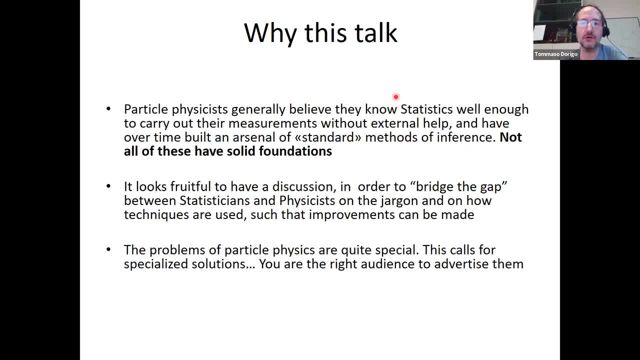 and physicists to attack these questions, but in general, it's good to have a discussion to bridge the gap on the jargon and on how we use the techniques, because this is an evolving field so that we can actually look forward to having improvements. 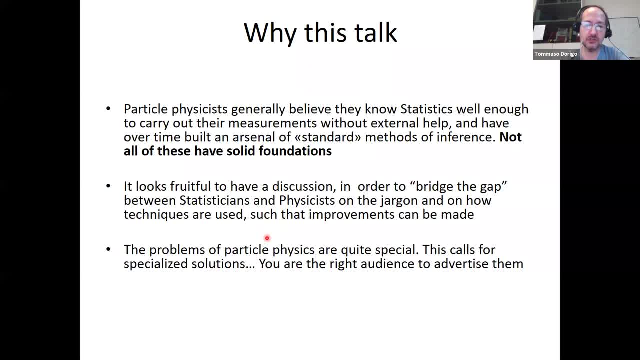 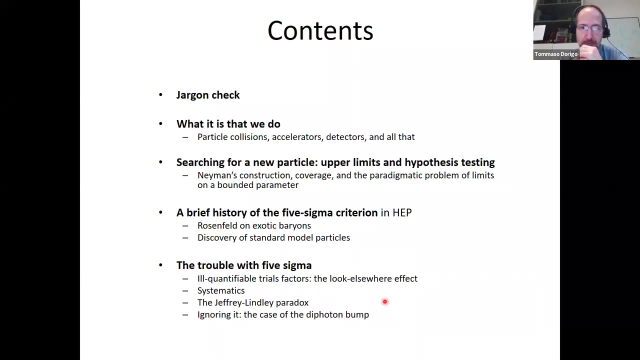 Indeed, our problems are quite special. so this is the right audience for me to advertise some of these techniques and see if we can go further. So the contents of today's lecture talk, call it as you like- is: first of all, we'll do a. 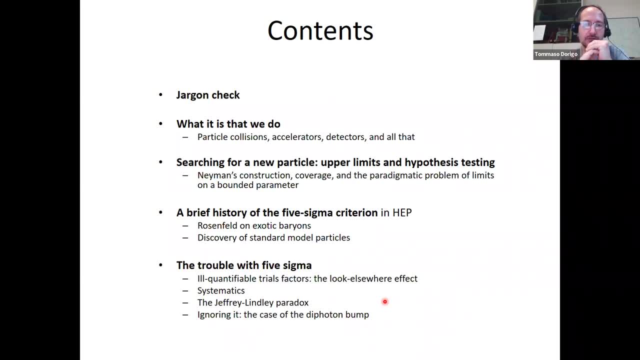 jargon. check to be on the same page with the way I'll talk about things. I have sort of interacted with statisticians over time so I can sort of speak the language. but well, you should also know how physicists typically discuss these things. 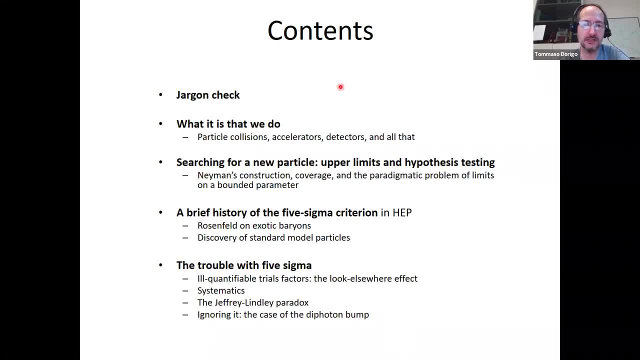 So we'll go through very quickly what we do in particle physics: measurements in these big giant machines, particle accelerators, and in particular how we search for new phenomena at the very small scale, Small distance scales. So we search for new particles and we, if we don't find them, we set upper limits on. 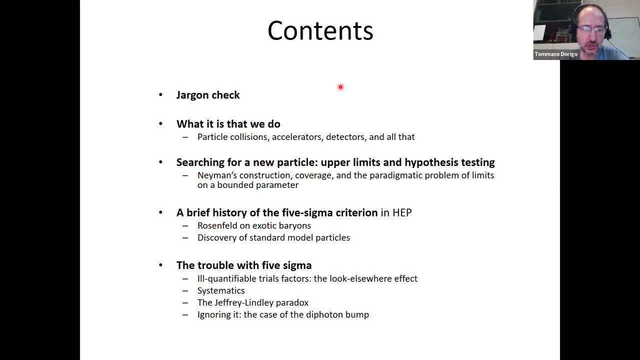 the parameters that describe their existence. So we'll discuss this Neymar's construction, I'll remind how we use it, at least, and some issues connected with the use of these techniques for our problems, And then we'll go through a brief history of. 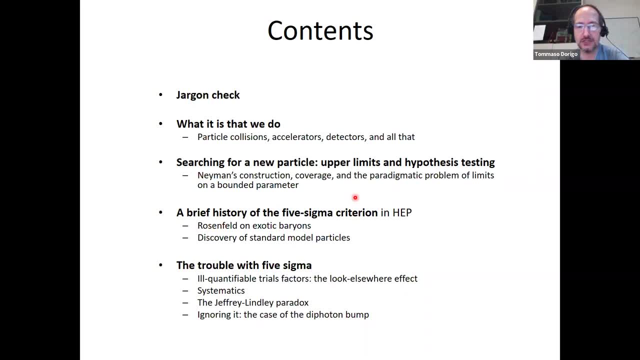 Okay, Okay. So let's start with the first question. So we have a criterion which is used in energy physics practice to decide whether we can go out and declare that we've found a new particle or phenomenon. We have this five sigma criterion, basically a type one error rate of 310 to the minus. 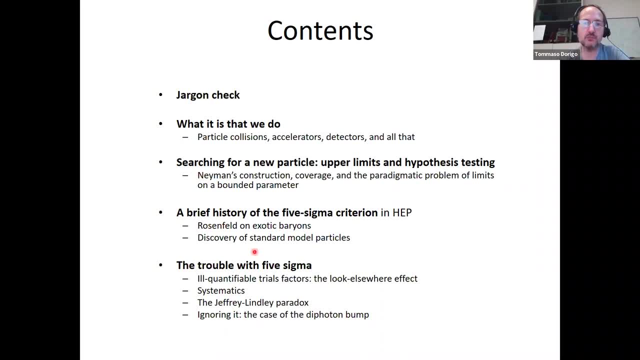 seven, And we'll see where this was born and because it's important to know what are the roots, And then we'll see what the trouble with this is, in particular on certain aspects. And okay, I think this will give me a chance to give you the flavor of the kind of business. 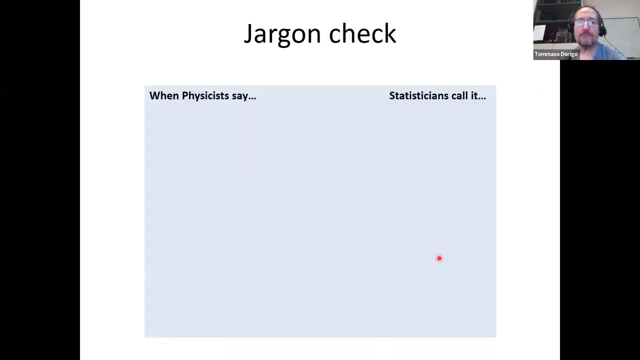 we are into. So a jargon check. When we physicists say determine. what you really should hear is that we are saying that we estimate the parameter, okay, but we say we determine it. And when we say we estimate at least experimental physicists. 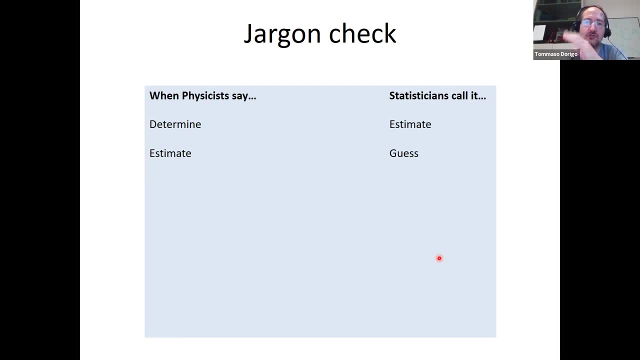 It's more of a. You should hear that it's more of a guess. So I estimate that this nuisance parameter is in this range. it's a guess, okay, And the observable space? that's how we call it. it's what you call a population. 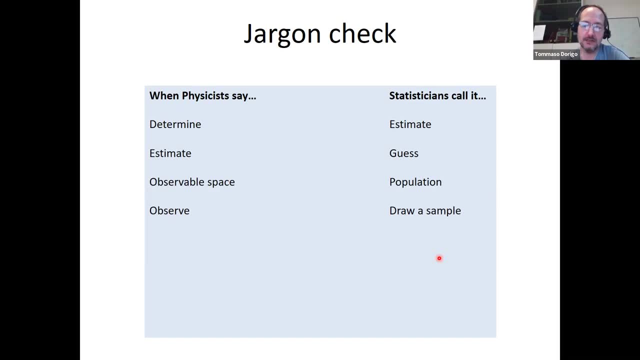 And so when we say we observe something, you would say that you draw a sample. An event or a data is what you in fact call a sample. And when we talk about, When we talk about uncertainty, we are not talking about our near future in this world. 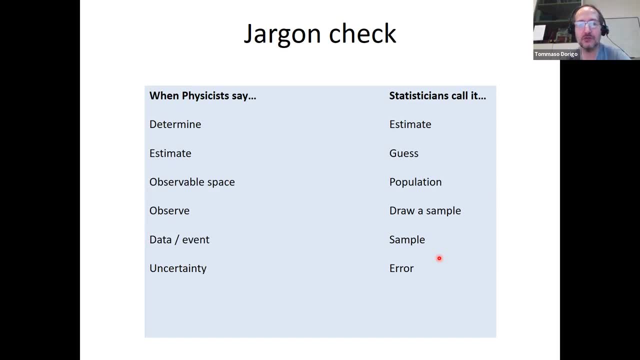 but we talk about really what you would call the error on the estimate of a parameter, for instance. okay, So we talk about the systematic and statistical uncertainty, But when we talk about error, unless we are talking about type one error rate or mean, 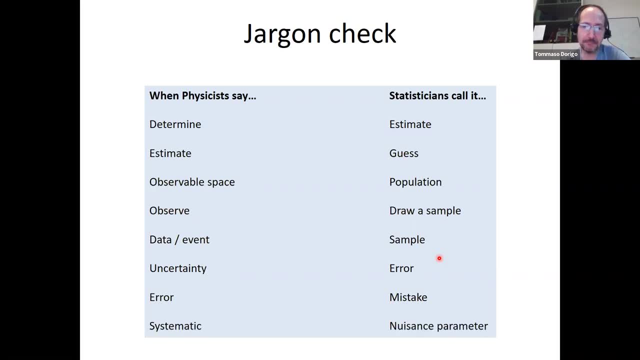 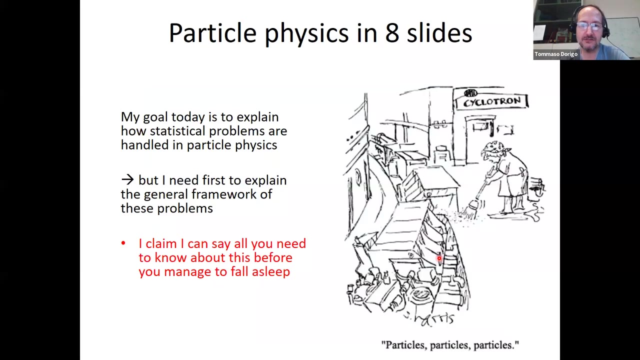 squared error. we really mean that we have made a mistake, And systematic uncertainty for us is what you would call a nuisance parameter. okay, So this is something that we should keep in mind when we have to discuss among physicists and statisticians. So the goal today is to talk about particle physics, measurements and searches. 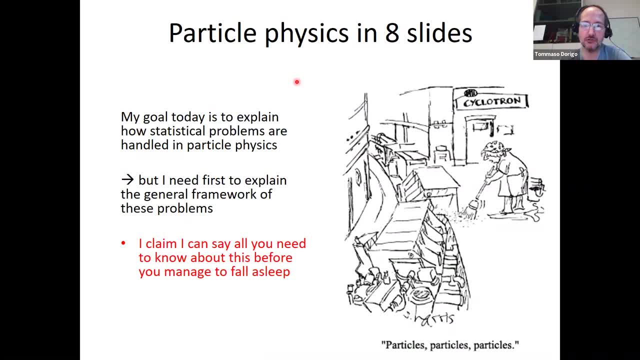 And so I think I need to give you a crash course in that and see if I- Let's see if I can make that in a reasonable amount of time. Okay, Okay, Let's see if I can make that in a reasonable amount of time. 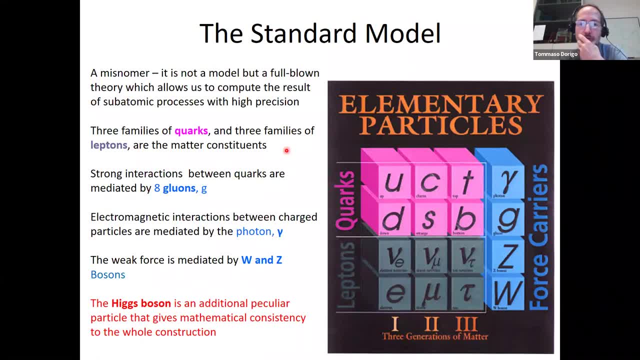 So we have a model which is actually a full-blown theory- a pretty good theory, I would say- that allows us to compute through the basic fundamentals of the theory of particles: particle fields, the result of subatomic processes with high precision. 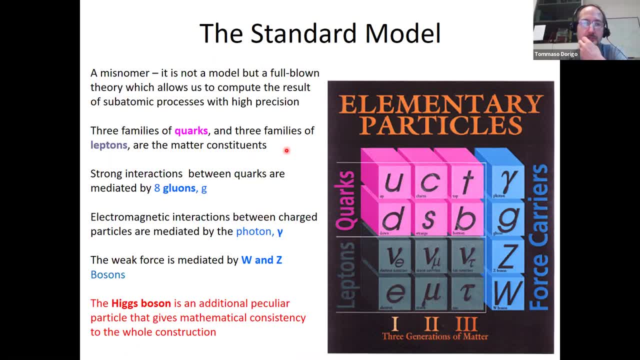 So we collide particles and we know what comes out. We know the probabilities, okay, And by doing these experiments through The last 50 years we have discovered that matter at its innermost scale. it's made of quarks that are constituents of protons and neutrons that make up nuclei of atoms. 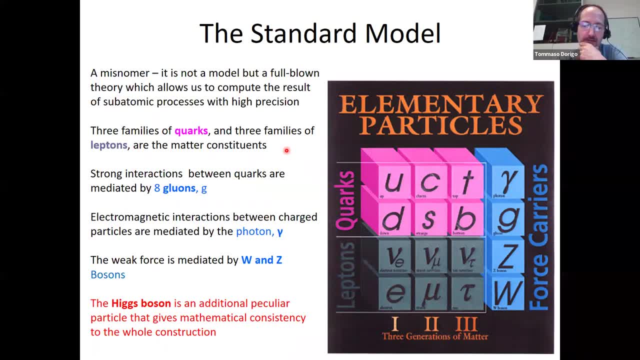 And there are three quarks in each: proton and neutron. In fact it's not just three, It's a sea of these particles that come into existence and disappear. And then there are three families of leptons- this down here, to which the electron belongs. 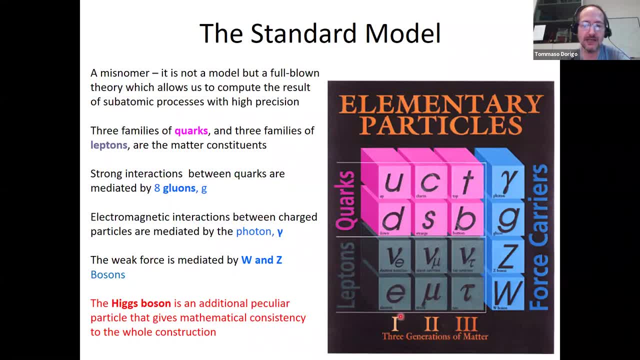 So the electron As we know it is a constituent of matter, but there are other fancy particles that behave similarly to the electron, and also neutrinos that are part of this lepton family. And then there are interactions, Force carriers are mediated. 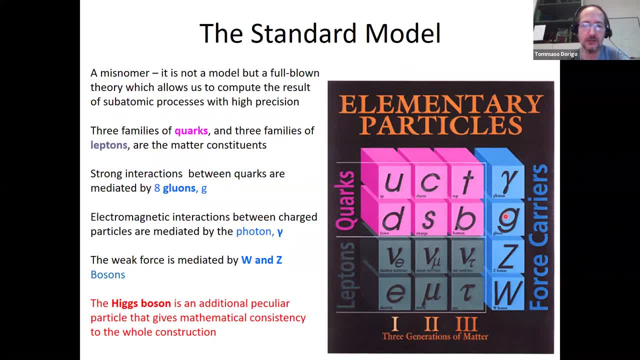 Forces are mediated by the exchange of gluons that are keeping the nuclei together, by the photon that gives us the electromagnetic interaction, and W and Z bosons that are important for fusion processes inside. And then there is one other particle that is called the X boson, which was predicted. 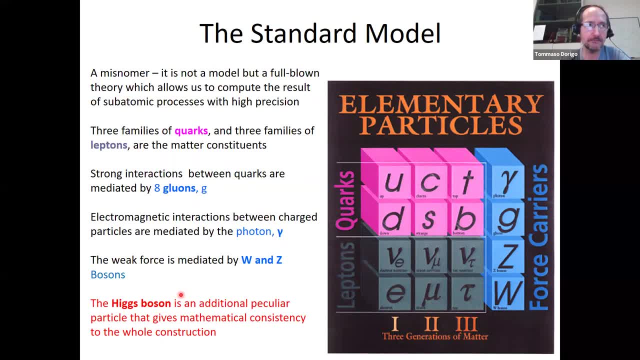 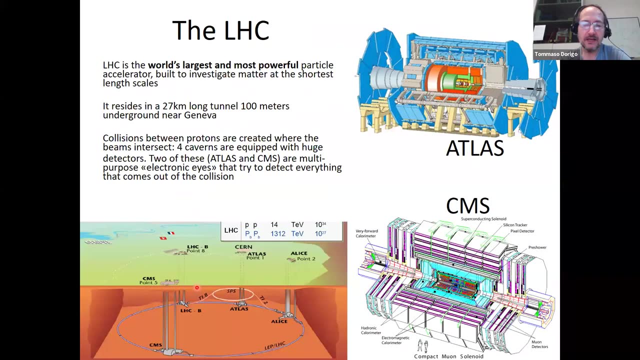 over 50 years ago now- 50,, yeah, in 1964.. So 56 years ago now- and was discovered in 2012 by the Large Hadron Collider. So this is the picture, okay, And in fact we have this large machine, which is a 27 kilometer long tunnel that is built. 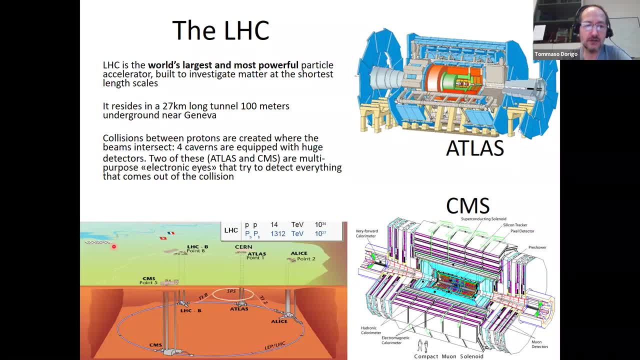 100 meters underground Near Geneva in Switzerland, which is instrumented along the ring by four large experiments. You see, these are humans on the scale that allowed to take snapshots of the proton collisions that happen at their interior 40 million times per second. okay, 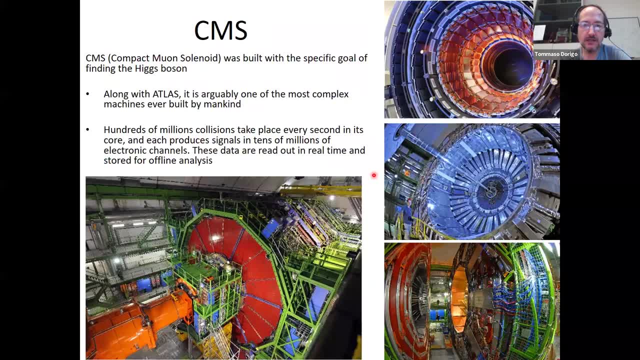 So these are gigantic endeavors. Here are a few pictures of the CMS experiment to which I belong. It's 350 meters long. It's a 1,000-strong collaboration that built this experiment and operates it. I argue that it's arguably, yeah, one of the most complex machines ever built by humankind. 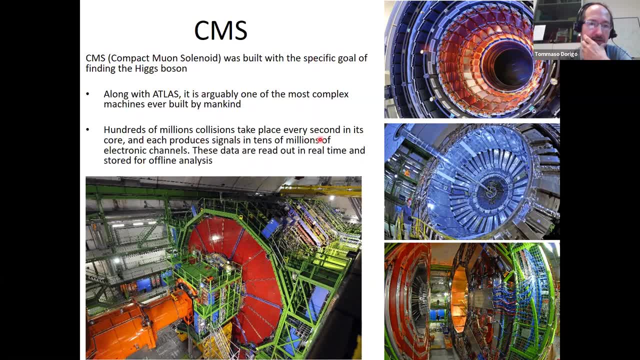 Hundreds of millions of collisions take place every second, and each of them produces signals in tens of millions of electronic channels. We read them in, we recognize the important features of the event, we store them and we analyze them and do inference. Okay. 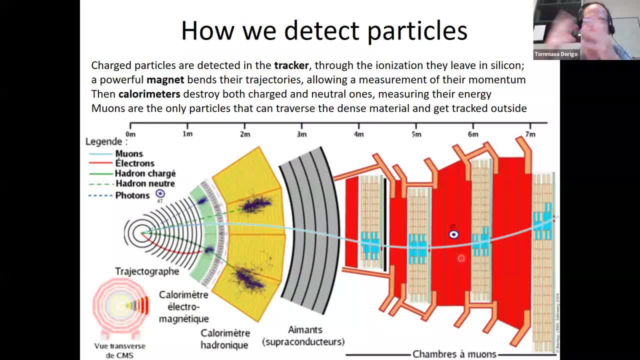 How do we detect the particles? and there's thousands that come up out of these collisions every 40 million times a second. So the particles that have electric charge are bent by a very strong magnet so they create curved paths And then, and by measuring how curved the path is, we know the energy of these particles. 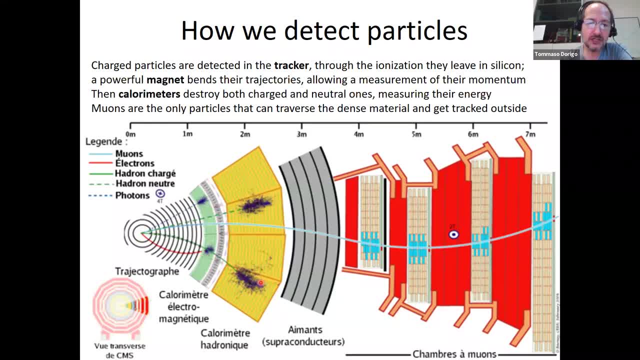 And then particles are destroyed, And then by interacting with dense layers of material in what we call calorimeters, so that we measure the energy also of particles that are neutral and didn't leave a track in the inner tracker, which is made of silicon sensors. 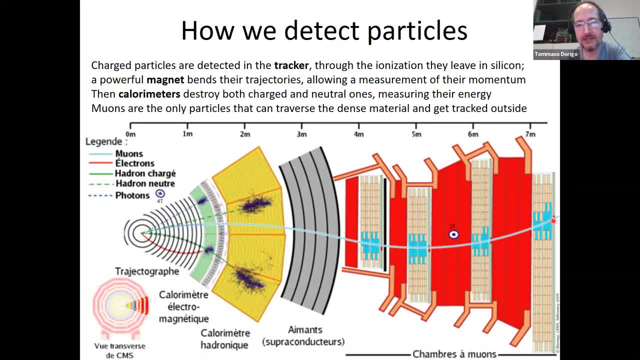 And then there are muons, that are these heavier brothers of the electrons, that can actually travel outside of these dense layers of material and get detected outside. So we reconstruct their tracks, So we're determining the species of particles And we determine their four momenta, their direction and energy. 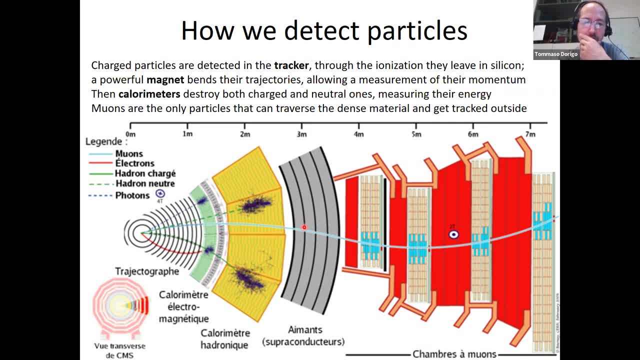 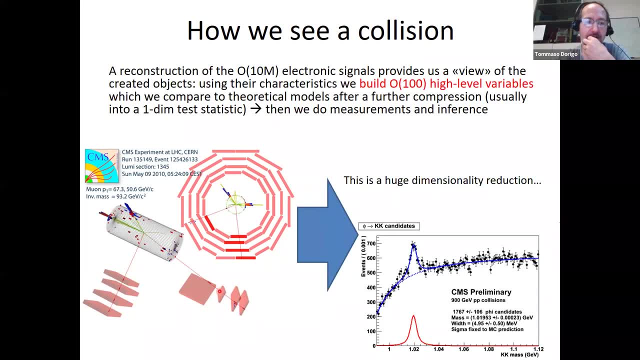 And this allows us to construct high-level features that tell us what really was it that the collision produced. So we have a reconstruction of the event, and then we have this fancy event displays that allow us to picture the amount of energy that flows in various directions. 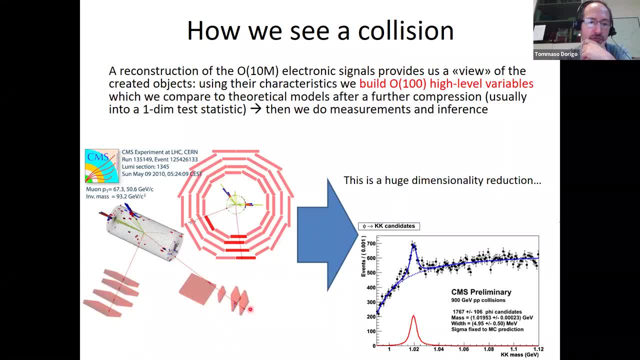 And here you see the tracks reconstructed of two muons, For instance in the decay of a, Of a heavy Z boson in this case, And then we do a huge dimensionality reduction. Well, there was already a large dimensionality reduction that brought from 10 million channels. 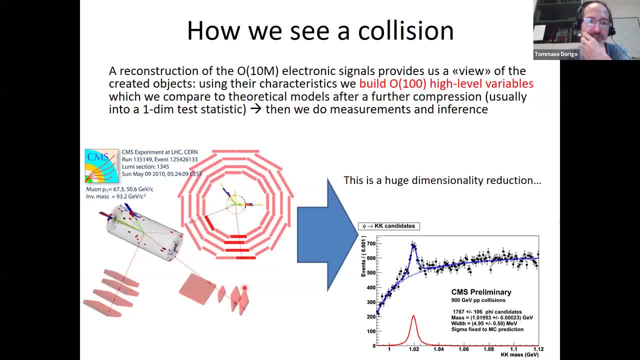 to maybe a hundred variables that describe the event. So there is a muon and it has this energy in this direction. There is a jet of particles with this other energy, and so on, And then we create another dimensionality reduction step that allows us to plot on a 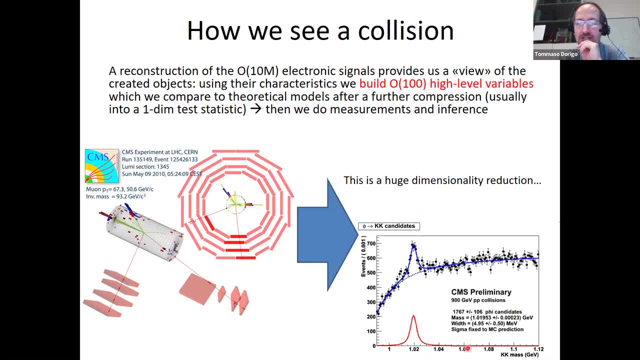 single dimensional histogram, For instance, the reconstructed mass that each observed event features if it gave rise to the production of a certain particle. So a particle has a definite mass, And so all the events that were in fact the decay of this particular particle will pile. 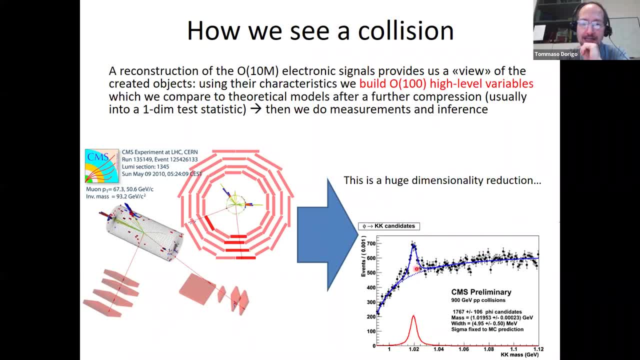 up with a Cauchy distribution at a certain mass value in the reconstructed mass distribution, While the background will have some More smooth shape, So that by finding peaks in this distribution we identify particles. We are spectroscopists As we were a hundred years ago: we still look for lines in a spectrum. 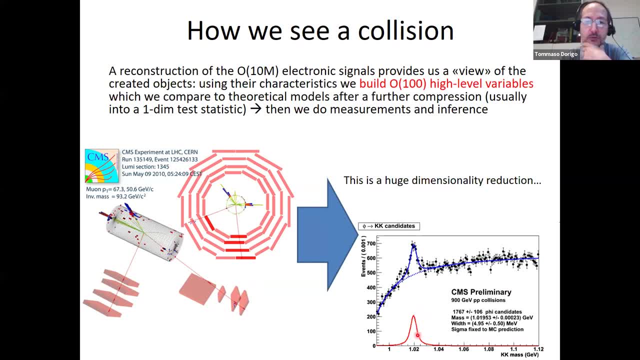 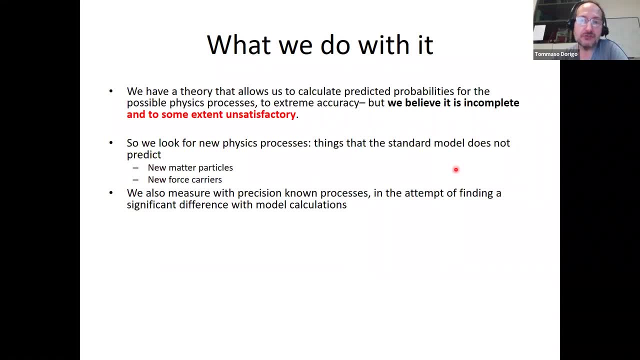 Only the lines are not so sharp. They are a little bit blurred by the experimental resolution. So what do we do with this? We have a theory, the standard model. It allows us to calculate predictive probabilities for the physics processes to extreme accuracy. 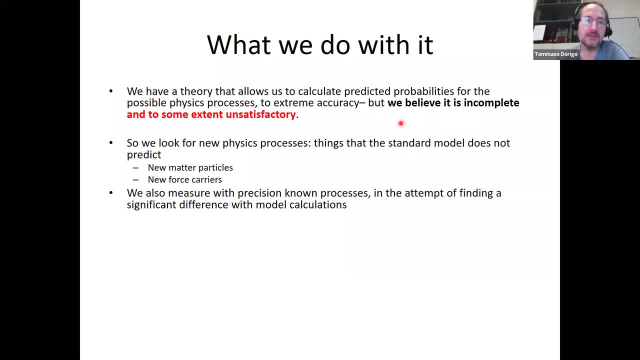 We believe that the standard model is: It's great, but it's incomplete And we want to see what's behind it. okay, So we look for new physics processes, other particles that may lie beyond that higher energy that we have not investigated in previous machines. 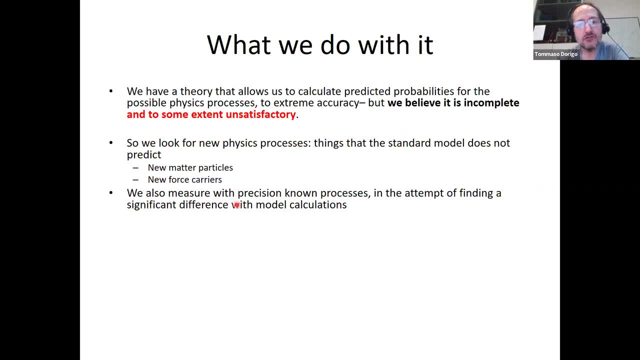 So we look for particles, new force carriers, And we also measure with extreme precision processes that are known, these probabilities that by colliding a proton I get a Higgs boson. I want to measure it as well as I can because 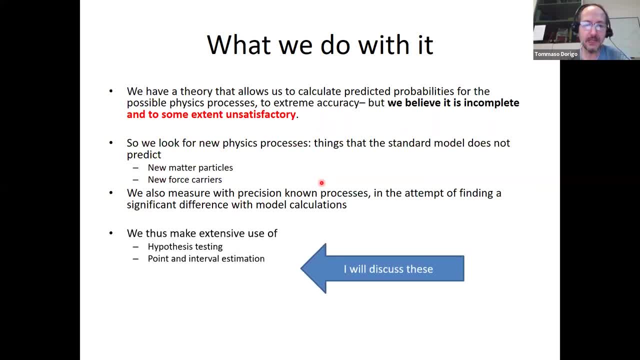 this will allow me to test the theory. So we make extensive use of hypothesis testing and point and interval estimation. We also do a number of other things, So we need unfolding techniques. We do dimensionality reduction, So we do classification or regression using machine learning tools. 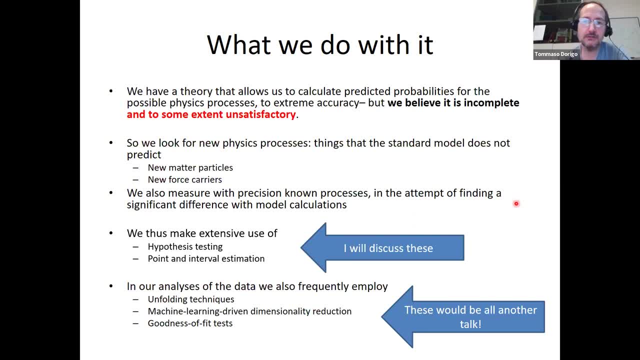 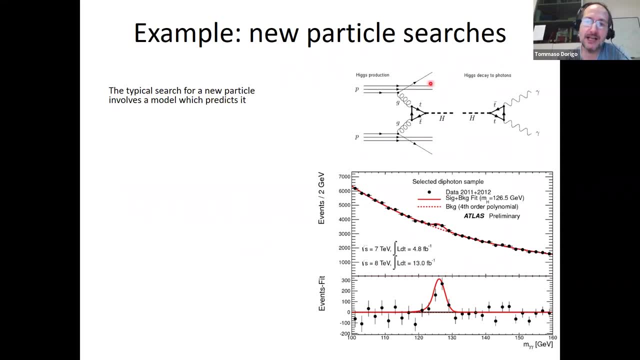 We do a number of things which we have no time to investigate today. So for a new particle search we use this funny function- Feynman diagrams, they're called- that describe what goes on at the subnuclear level. So you have a proton coming in, another proton coming in. they exchange particles, they create. 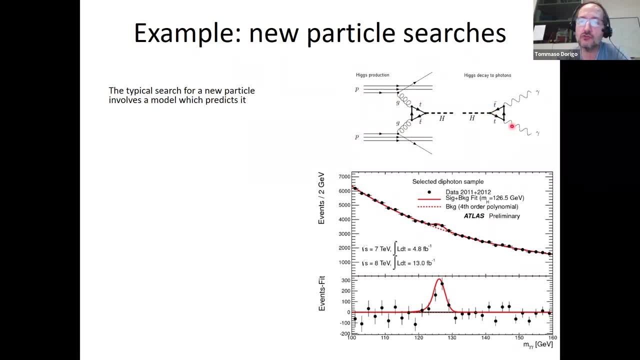 a Higgs boson and then this particle will decay and produce two photons that I can actually measure in my apparatus. So we have Monte Carlo generators that take in the theory and they can be plugged into simulations And then we get Artificial data that describe what we should see if we see a signal of the Higgs boson. 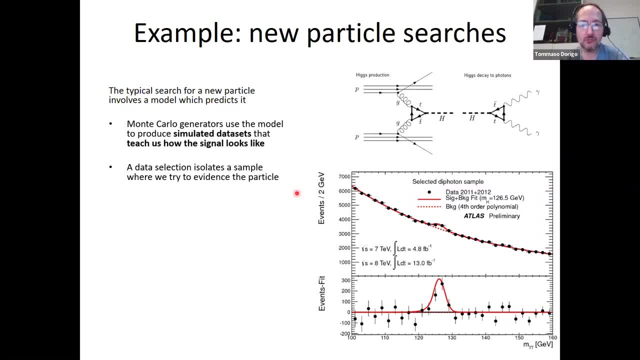 decay. And then we select the data and we try to evidence the particle by creating, say, a histogram of the mass of the observed events where, if there is an accumulation at a certain mass, once we subtract the background we can see that there was a signal. okay, 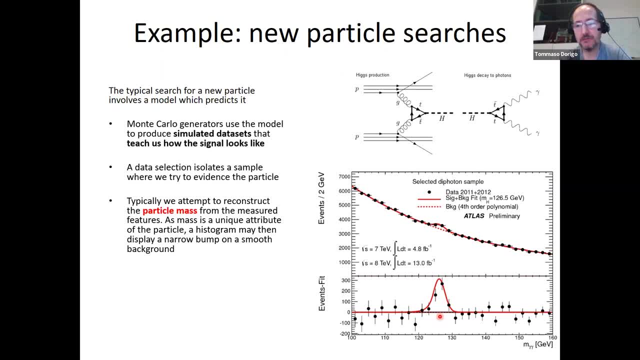 So this is basically well, not 100%, but I would say more than 50%. We do a test of hypothesis which allows us to derive the probability that we saw this data, given the fact that, I may say, there is only background. okay. 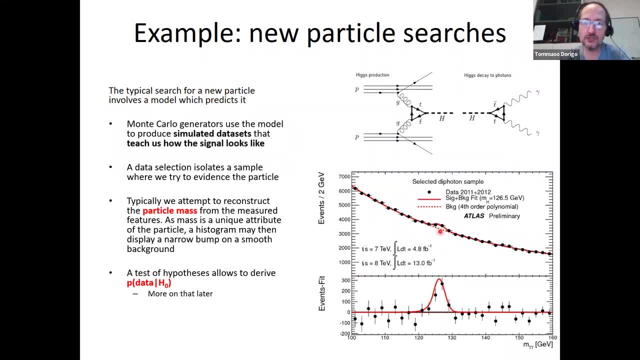 So this might be a fluctuation And if the probability of a fluctuation, well, the probability of the data, given only a background model, if this is very, very small, below 310 to the minus seven, we claim that we have. 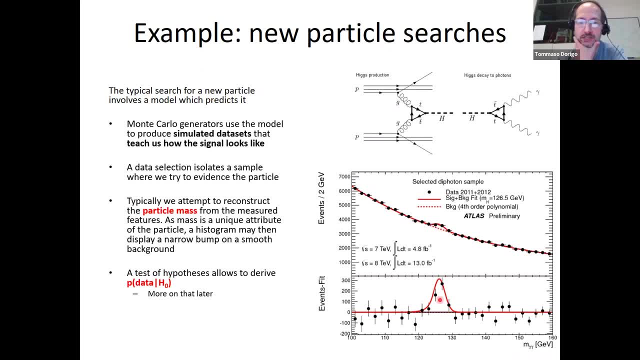 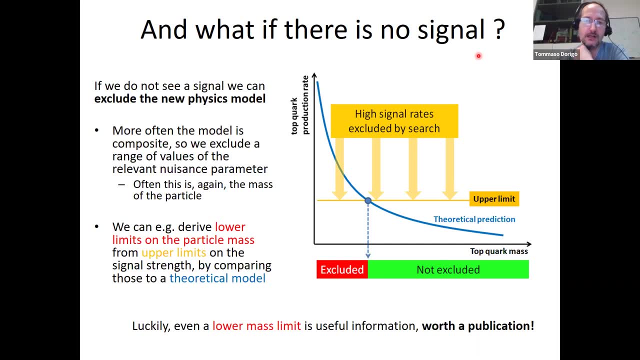 discovered a new process. Okay, So we'll discuss this more in detail later. If there is no signal, we can rule out theories. How do we do that? Well, if there is a distinct theory that says there is a new particle with a certain mass, 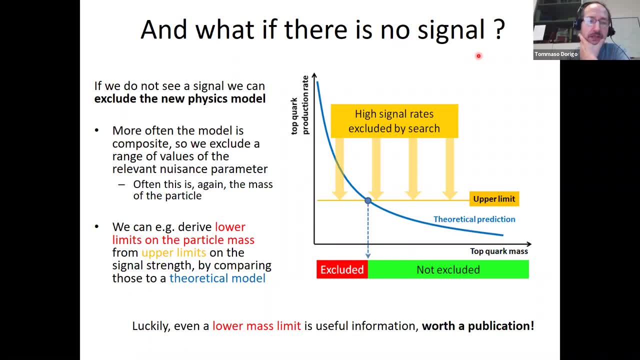 we go, we don't find it. we say the model is wrong. But more often the model is composite, so there is a nuisance parameter, in fact, that the mass of the particle is not known beforehand. So we investigate a range of possible values of the mass. 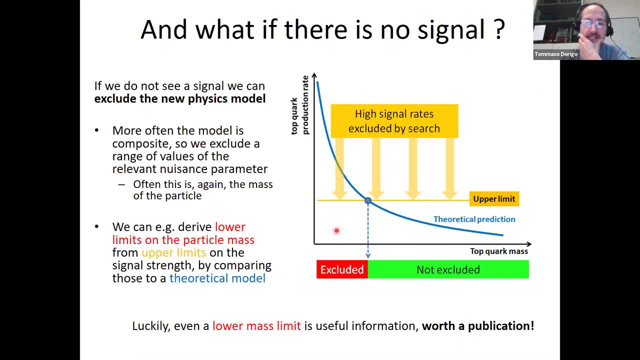 And we can do inference in every point of the mass and say, well, I can limit the rate of this process to a certain value because I didn't see more than, say, 100 such decays. If there were more than 100 such particles in the data set, I would have seen an excess. 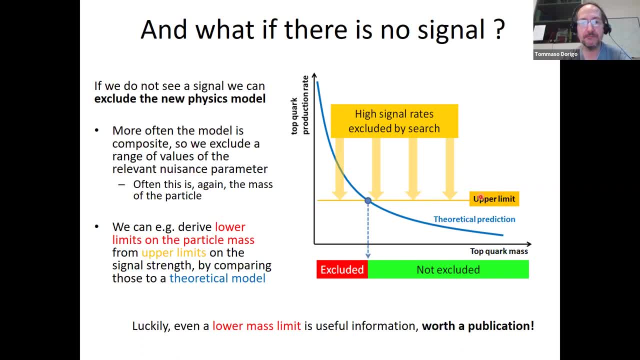 But I didn't. so I have an upper limit on the signal rate And then I compare this limit to a theoretical limit. Okay, So I have a vertical curve which says that it is more likely that we produce many particles if they have a small mass and it is more likely that we produce few particles if they. 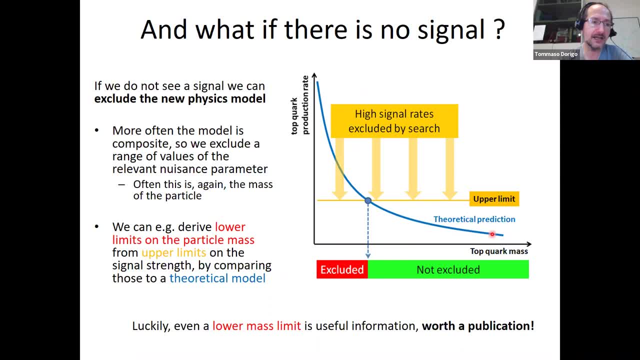 have a large mass, And this is basically due to the fact that the higher energy processes are less likely to take place in our collisions, And so we can say, okay, I set the limit here. So what this means is that I can exclude all values of mass below this value. 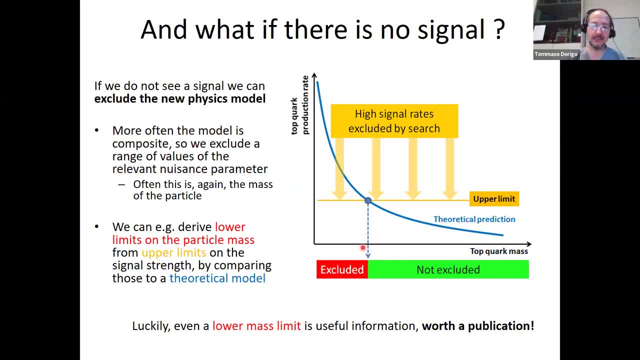 So this tells me The model may be still good, but at least I can chunk off a parameter space part that tells if the theory is right that this particle must be heavier. And this is important input and it allows us to publish our results and get citations. 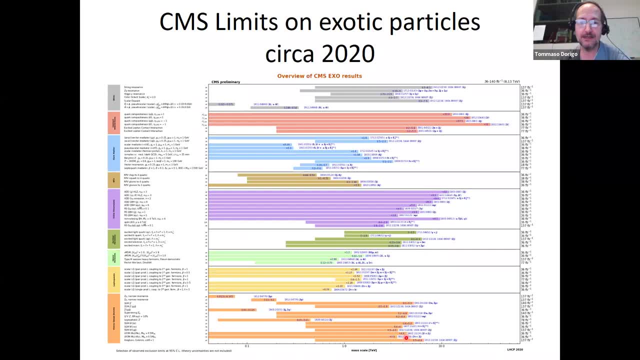 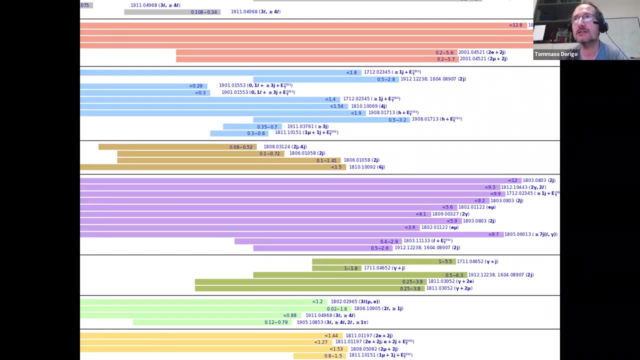 Okay, In fact, we do most of that. You cannot read this graph and I don't want you to read this graph, but if you did, you would see that, In fact, each, Each investigated model has a range of exclusion where the model was tested and was not proven. 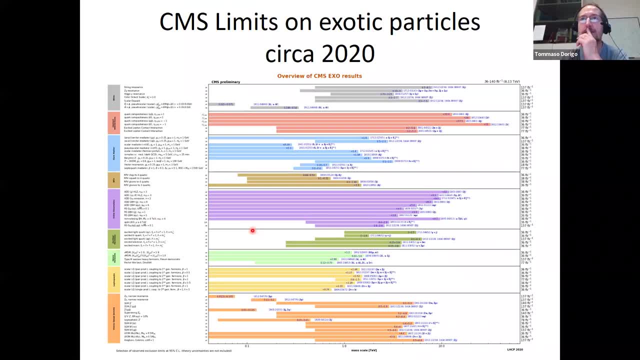 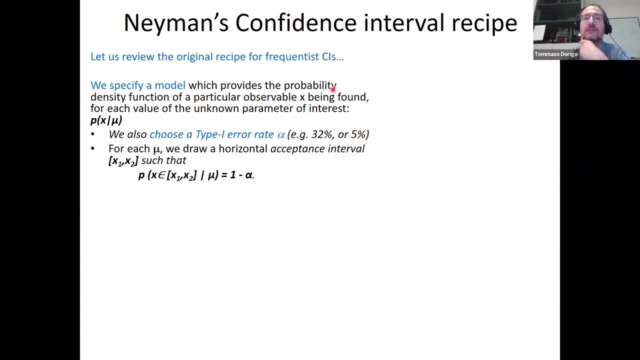 correct. So this is generally the business that we do in particle physics experiments: We rule out theories as a function of the theory parameters. okay, So how we do it is by using the deriving confidence intervals, And so there's an old-fashioned way of doing it. 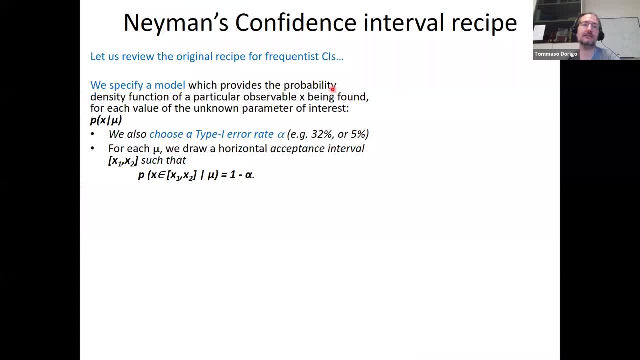 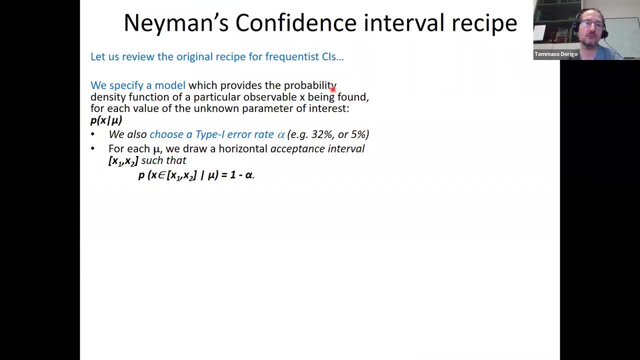 We have better ways- Well, better, I wouldn't say better- different ways to do it. But let's give a look at what Neyman's construction is, because it's relevant for a couple of points I'll make later. So you know, we specify a model which provides a probability density function that a particular 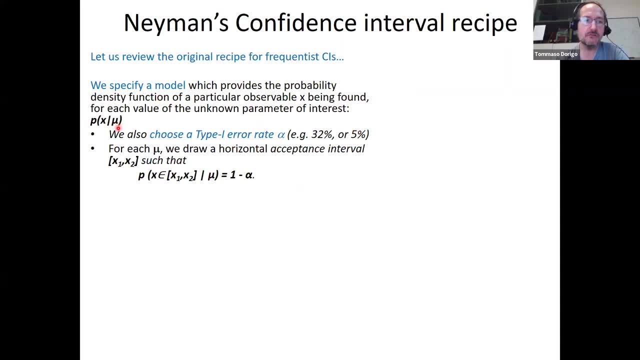 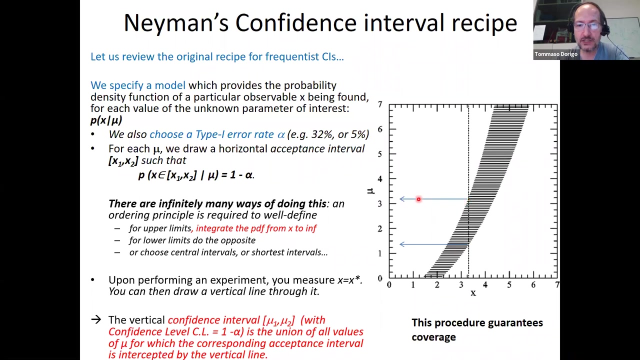 observable is seen given a certain value of the relevant parameter of interest, mu, And of course we specify a type one error rate And then for each value of the true value of the parameter, we draw a horizontal acceptance interval in a two-dimensional graph such that the probability that if mu has a certain value, 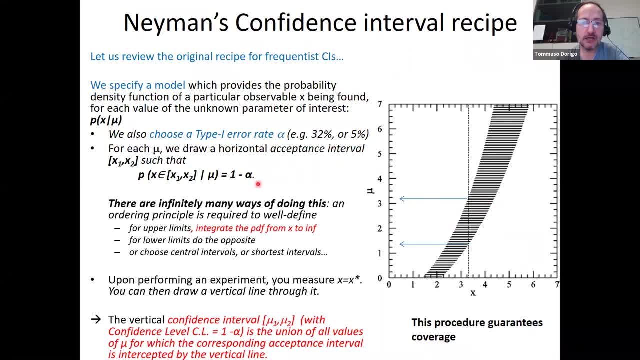 I will find x in a certain range is given by one minus alpha. So I have to decide how to order the values of x that I am integrating So typically. I will construct central intervals such that they cut half of the type one error rate on each of the sides of this. 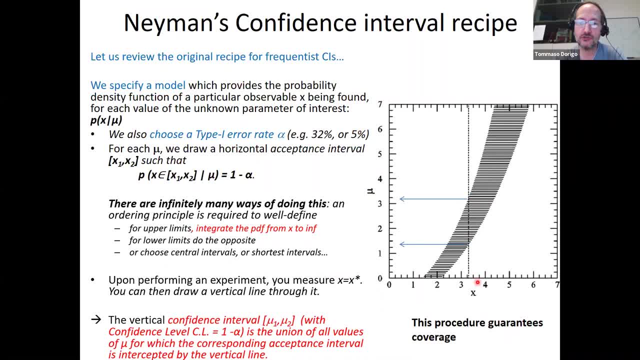 And this will create two curves of mu versus x. And once we do that and we actually perform the measurement and find the value of x, we can construct a vertical line and cut away and see the values of mu which are compatible with the observed x. 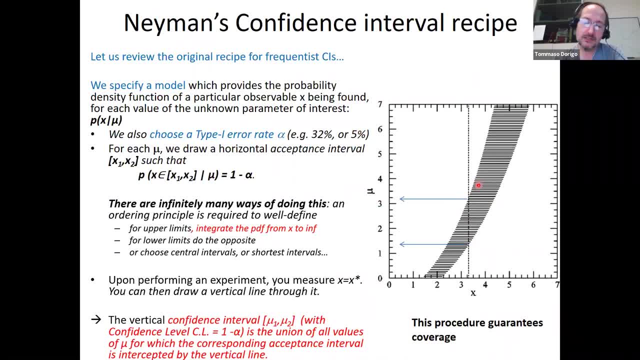 So I can extract. I can extract an interval for mu, But in some cases I will not be sensitive to specific values of mu and I can only derive upper limits. So to derive upper limits, I will have a curve, only one curve, which is derived by integrating. 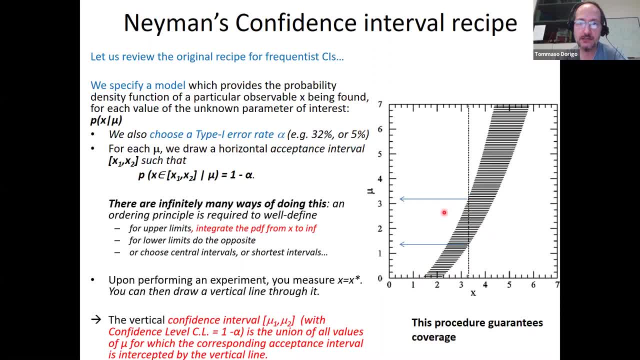 these PDFs horizontally from x to infinity, and then I get this curve. Okay, Anyways, this is Neyman's recipe and it guarantees frequentist coverage. So the average is very important for particle physicists because we want to have a way to 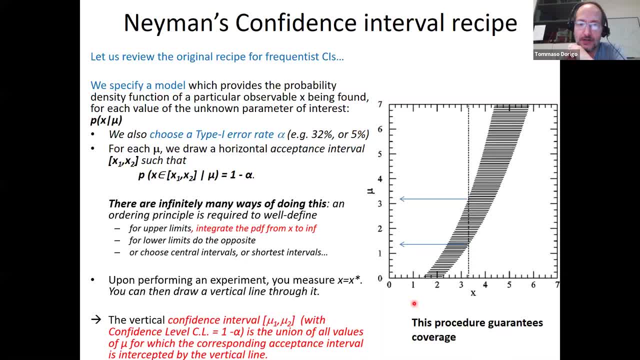 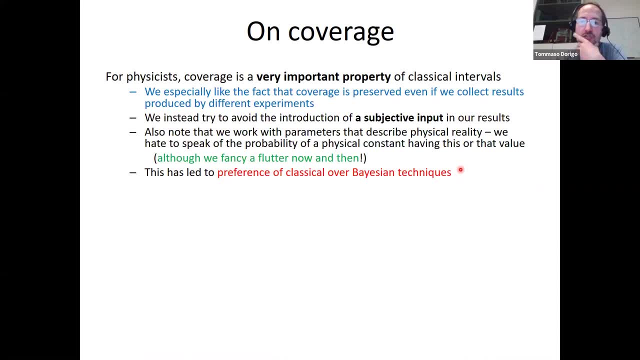 correct to be sure of what we are talking about in terms of the probability of the phenomenon, Since we are measuring physical constants of nature which we believe have a defined value, although we don't know what it is, We can hardly speak of the probability of a physical constant to have a certain value. 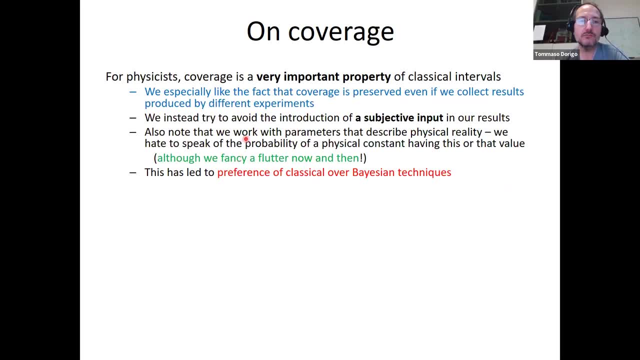 although we don't know what that is. So we tend to be doing our business in frequentist way, So we tend to like coverage as an important property of our measurements, Okay, And we also try to avoid subjective inputs in our measurements because we try to picture. 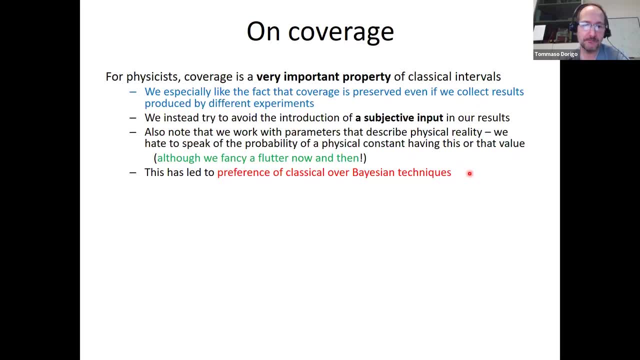 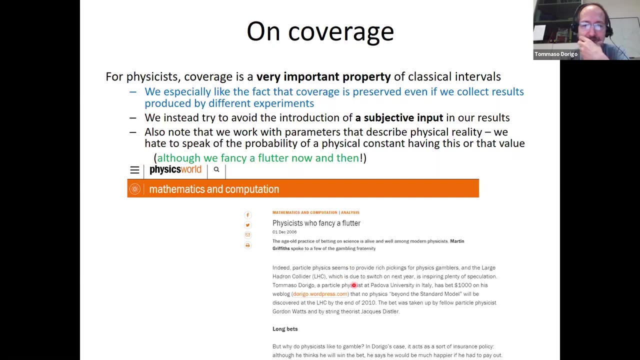 the way really nature works, and this should be objective. So this has led to preference of classical measurements. Okay, So, so this is the function of the, the function of randomness, This is what what we would call a frequency of the frequency of the. 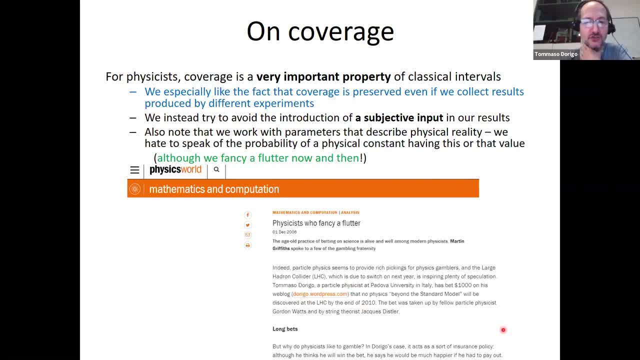 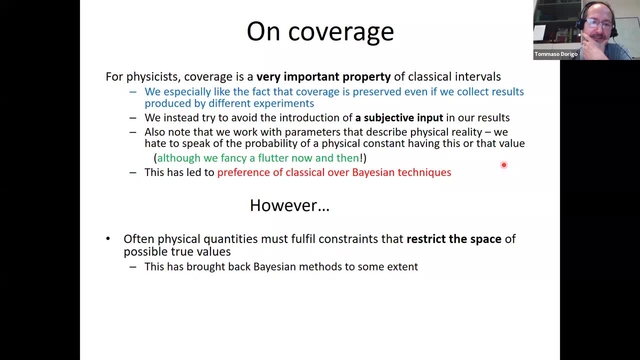 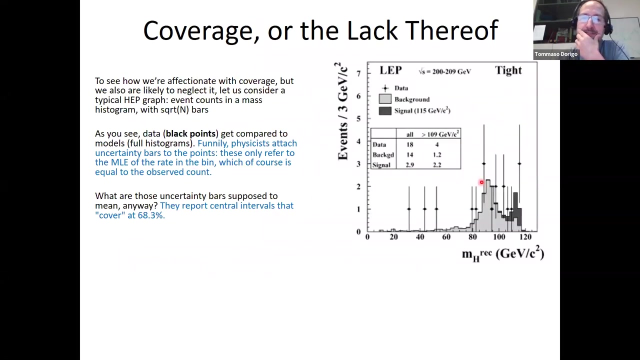 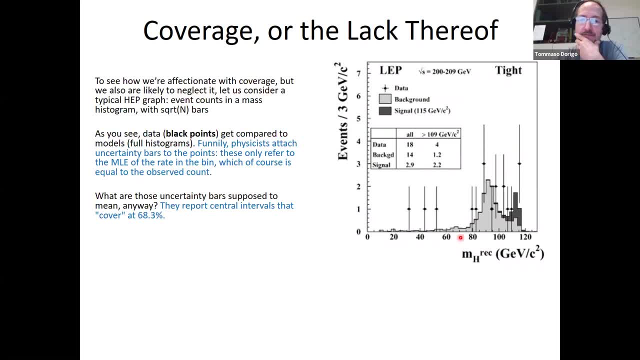 it. I will take a chance to show you a graph that was very important when the X boson was sought for in an experiment prior to the LHC, which eventually discovered it. Here in black, you see that the model that included the Higgs boson would predict that there would be a little bit of events. 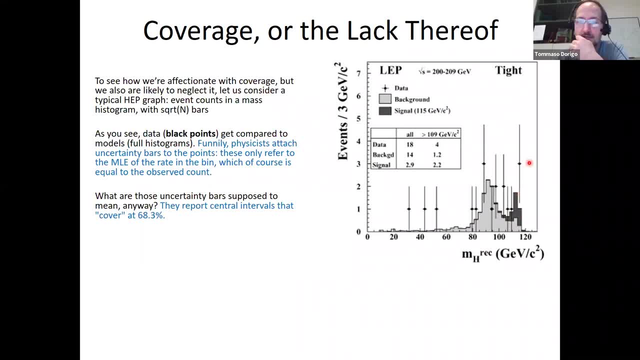 at the high end of this mass distribution And the fact that they have observed a few events in this region led to them claiming that they had a three sigma evidence for this particle. But I'm taking this graph. we will discuss more about the Higgs discovery later, but I will take this graph only to show. 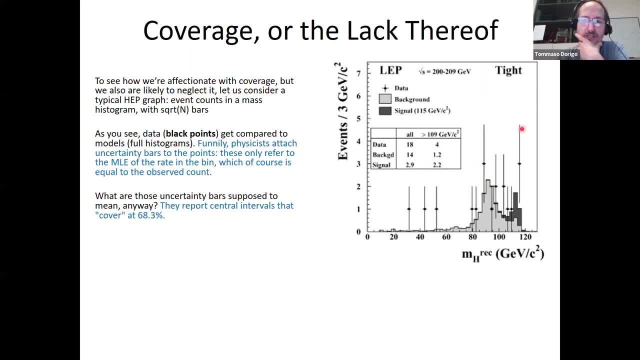 that these people in the 90s- well, this was 2001, I think- they still plotted these data points with uncertainty bars. So this means that you're doing two different things: You're saying how many events, you measure that a certain mass value and you're saying what your estimate for the maximum. 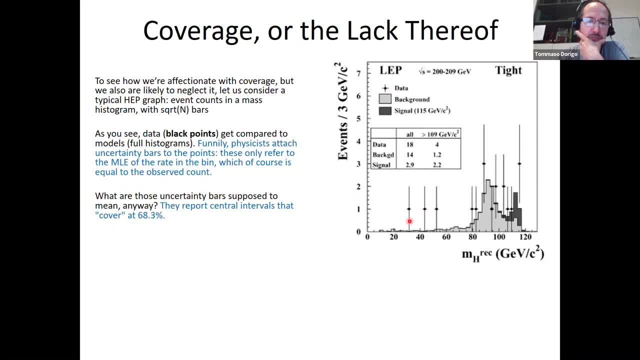 likelihood estimate of the rate in that beam is, and then you attach a vertical bar to the 68.3 percentile range of variation of that maximum likelihood estimate. But if you do that you immediately recognize here that they are doing one plus or minus square root of one or three times. 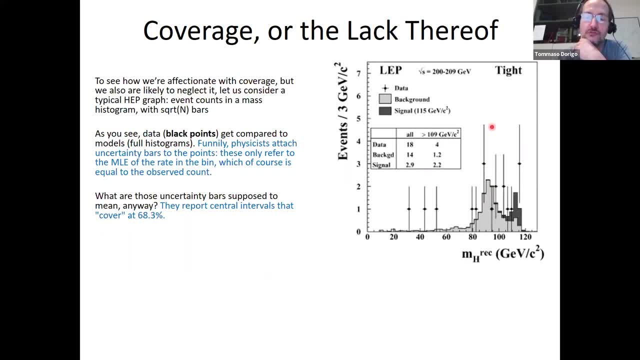 plus or minus square root of three. So they are taking the variance of the boson, which is the distribution these data are drawn from, but then they disregard the fact that for low event counts that you cannot plot 68.3 intervals that way. 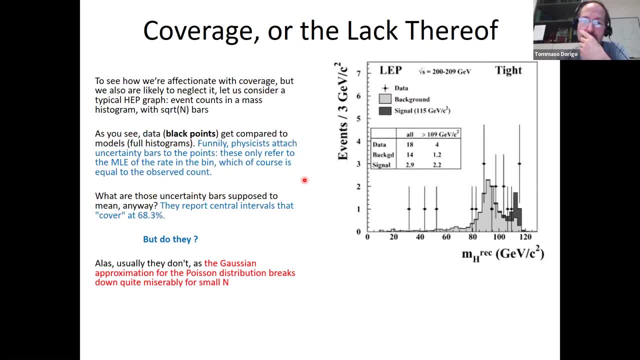 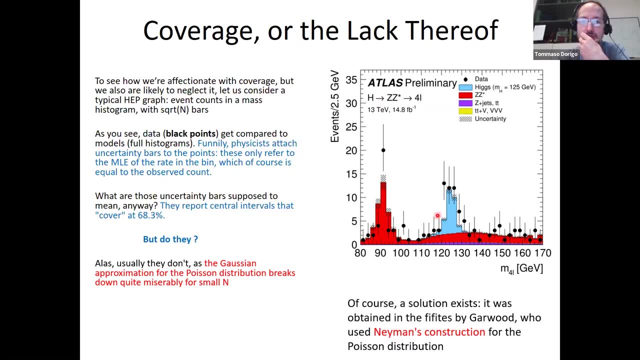 So the Gaussian approximation for the Poisson breaks down quite miserably in low energy regime, in low events regime In fact nowadays this is a graph of the Higgs boson peak found by ATLAS at 125 GeV. You see the signal is in green, in blue here, and you see that the error bars have. 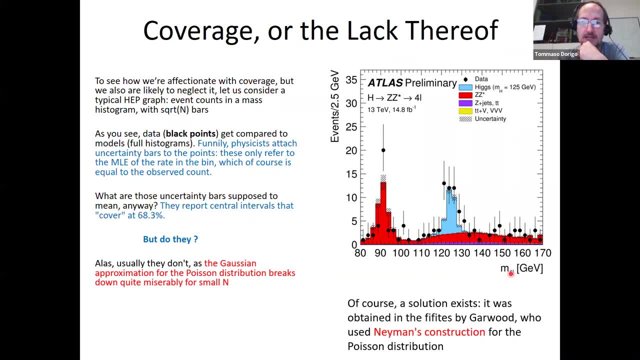 become asymmetric and they do cover, as at the required 68.3 percent confidence level, because they are extracted by inverted the Poisson hypothesis And this was done by Garwood in 1950 for the first time. So that was just a note. But the Neyman construction and the related techniques, 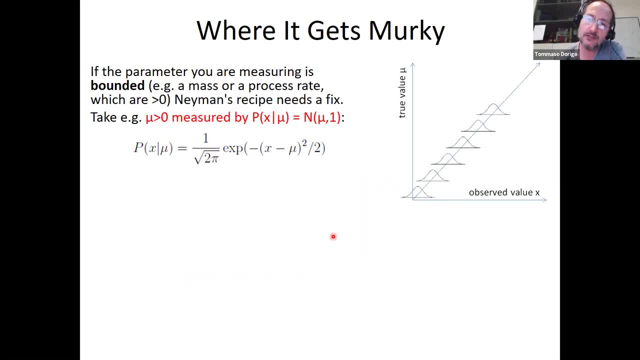 are somehow problematic in a kind of application that we usually, that we are in, we care about, And this is when the parameter we are interested in is bounded. So if it is positive, the Poisson problem is solved and it is perfectly aligned. Then we can examine this problem by. 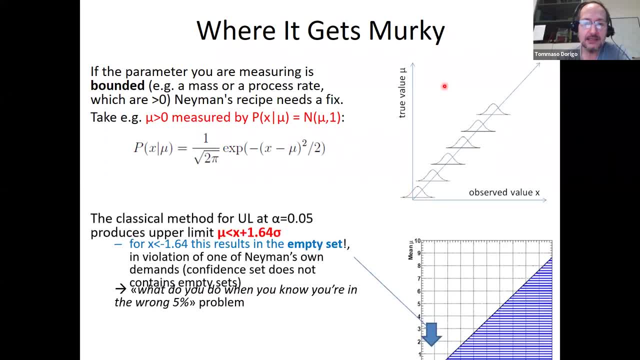 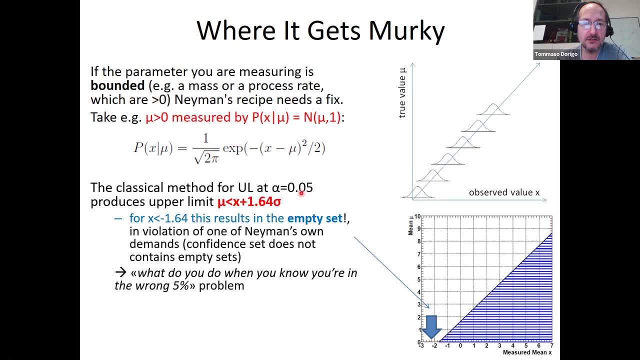 taking a normal distribution of our observable, so a Gaussian distributed measurement, And you immediately realize that Neyman's construction for this paradigmatic problem gives you upper limits at five percent confidence, type one error rate That are mew less than x plus one point sixty four. This is this vertical, this diagonal line. 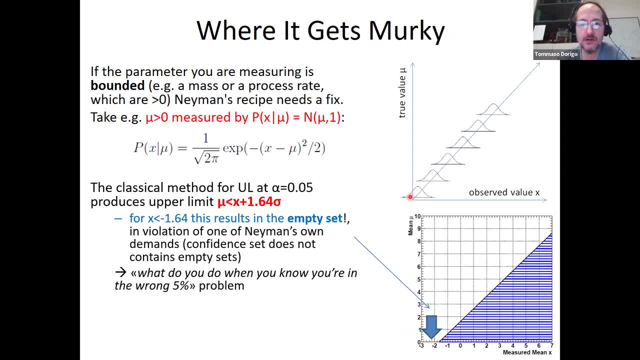 equals minus 2, which you can, because you have a Gaussian resolution- you are returned with an empty set. You don't know what to do in this case. Okay, so this is known by physicists. what do you do when you know you are in the wrong 5%? So it can be fixed? but 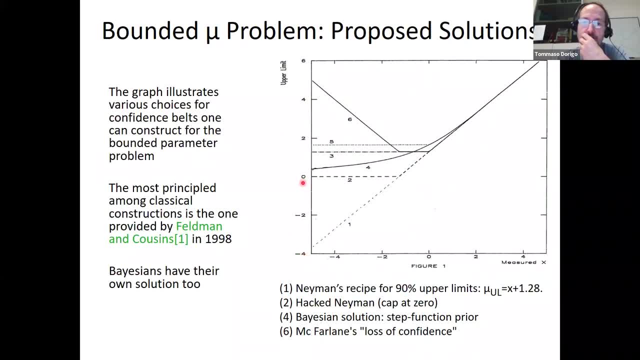 there is no general agreement on how to deal with it. In fact, several fixes are being proposed. There's Bayesians that have their own solutions. There's even a loss of confidence curve that says: if you really measure very negative values, that means that your measurement. 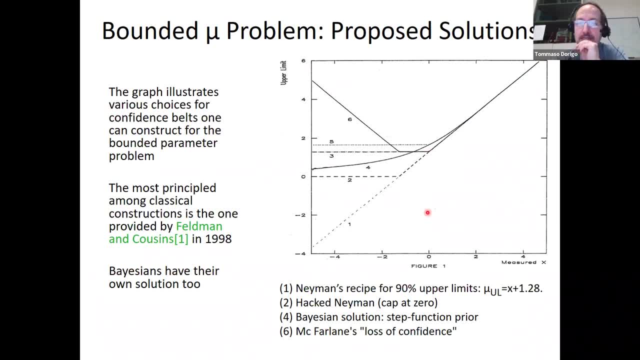 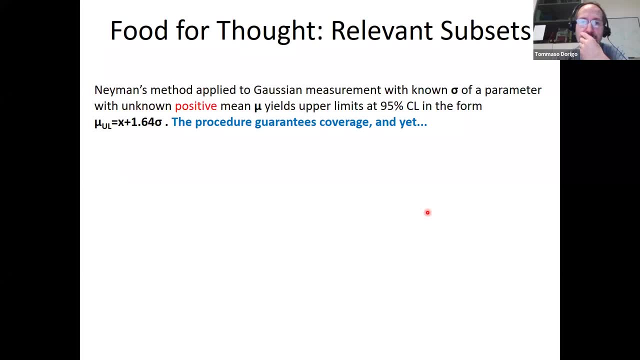 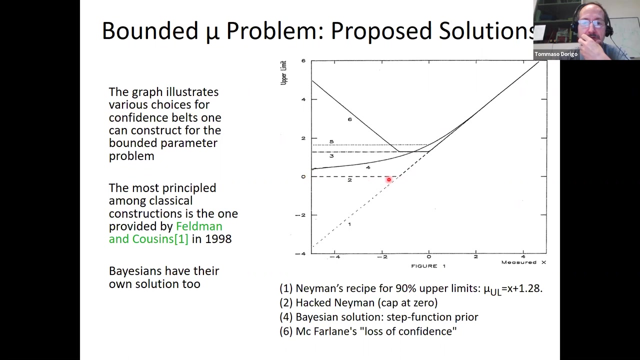 is bogus and you should increase your upper limit. So this is an active- somewhat still active- area of investigations on what to do, And I will even add that the procedure of Neyman, when you fix this upper limit, with saying that you put at zero the upper limit, if you 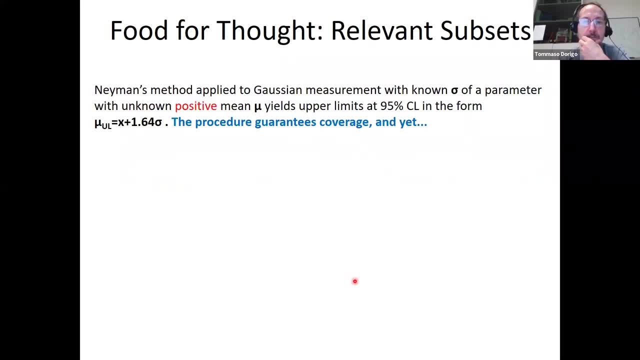 get negative, very negative x values it covers. but you can devise a betting strategy against it at nominal odds- so 5%, so 19 to 1, and be guaranteed to win in the long run. And this shouldn't happen, right? But you just choose a real constant k and you bet that. 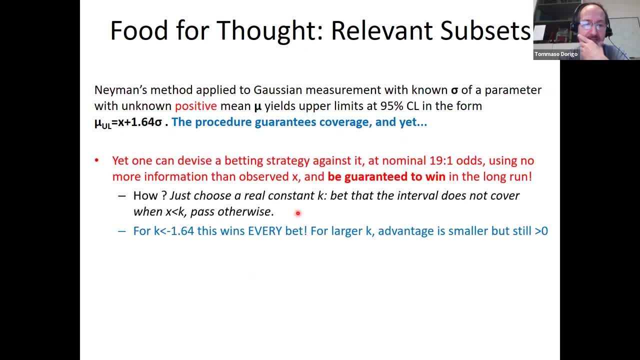 the interval does not change, And then you have a loss of confidence curve that says well, because notebook is not correct. So that's all about this. Okay, So with this, it doesn't cover when x is less than k and you pass, otherwise you don't bet, So you? 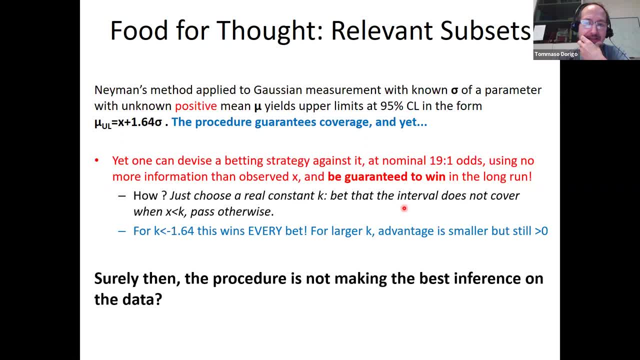 realize that if you can devise a betting strategy against a perfectly covering interval, there is something wrong going on, And in fact it has to do with the theory of relevant subsets, and there is a paper that discusses this by a physicist, Bob Cousins. This is has to do. 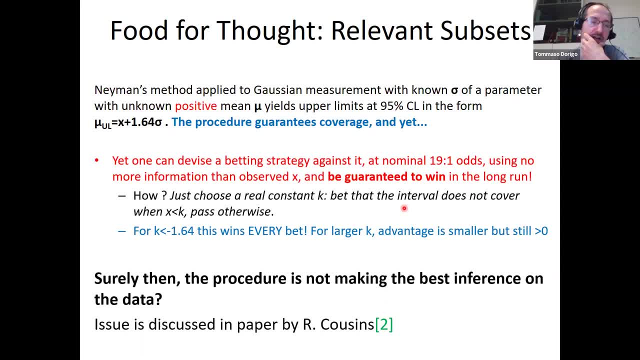 and in fact Cox devised a Gedanken experiment with two scales and you have to decide which scale to use to measure your weight based on the outcome of the flipping of a coin. One of the scale is more sensitive, and how do you define the uncertainty on the weight? So 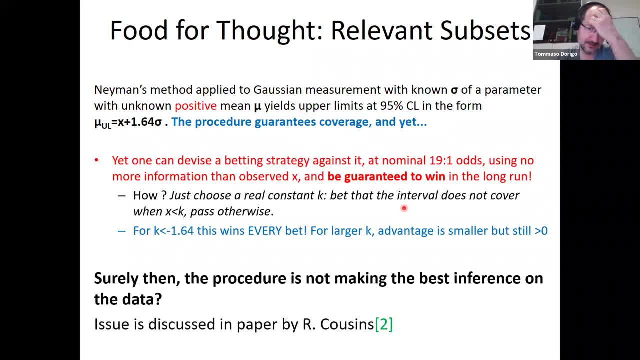 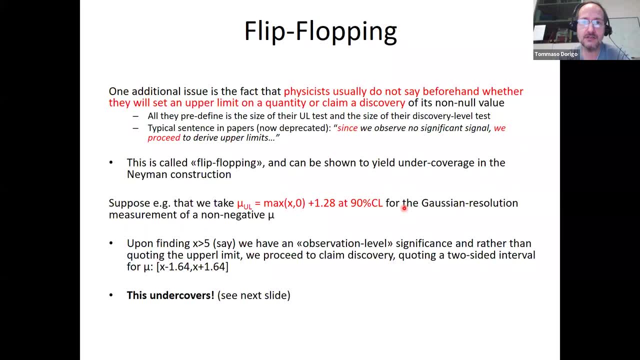 I will leave this here, but this is interesting, I think, and it highlights the fact that there are still some subtleties not completely solved in this area. And there is another thing called flip-flopping. that has to do with the fact that we don't decide beforehand whether we will claim. 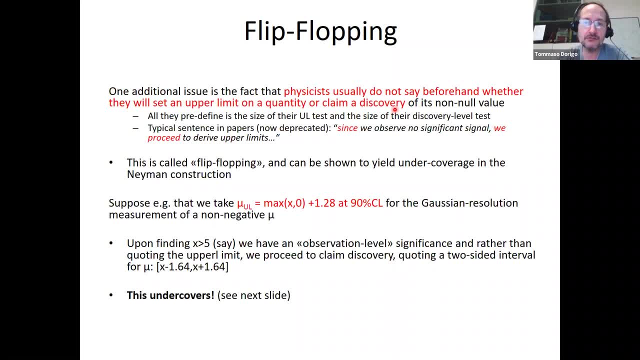 a discovery of a new particle, or put an upper limit on some parameter before actually getting the data, And typically this results in this awkward phrase in our papers: since we observe no significant signal, we proceed to derive upper limit. Then it means you are flip-flopping. 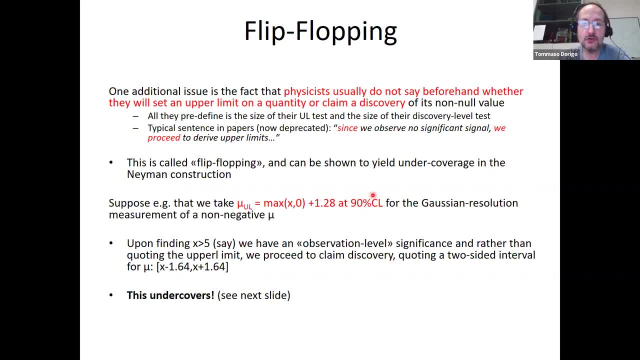 So suppose that we take again this paradigmatic Gaussian resolution measurement and fixed with this max x or zero at the very negative value of the x, Say that if we find a very large signal, then we put an interval around mu, while if we find x much smaller we put an upper limit, This property. this has the unfortunate result. 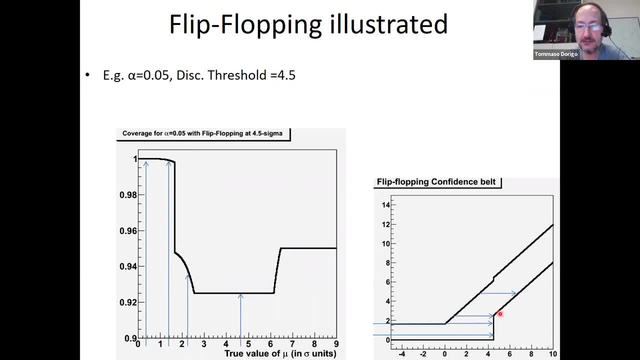 that the technique undercovers. because if you construct the confidence belt this way, you will find, and above a certain value you claim discovery and you set an interval over the measured value of mu, but below it you only set an upper limit based on a man's construction. then you 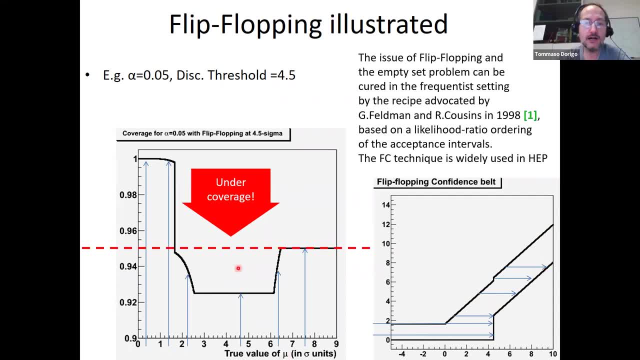 have a range of true values of mu for which you are under covering. Okay, and this is actually an issue. So we have corrective problems there. Another thing is, if you are giving mu this kind of corrected our papers, we don't say any longer, since we don't observe a signal. 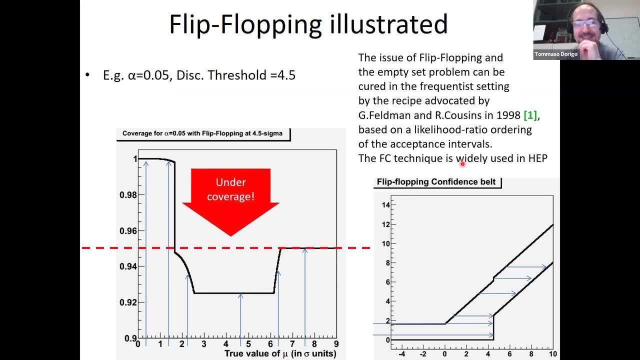 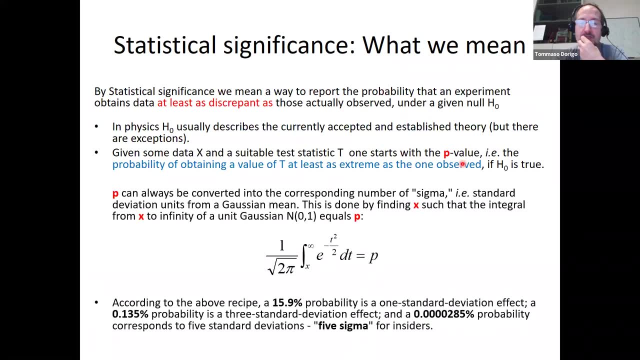 we put an upper limit, but we still do it. Okay, so it's kind of awkward. Okay, you certainly know what's the definition of statistical significance. It's based on integrating the tail of a Gaussian distribution, and this allows us to convert probabilities, p-values, into number of of sigmas. Okay, and we 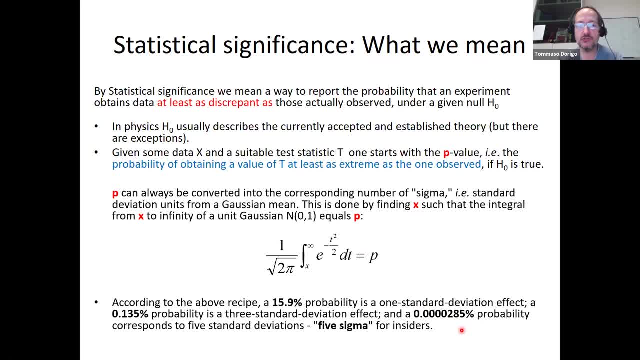 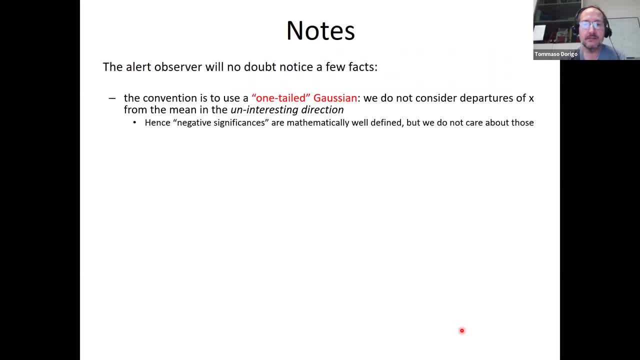 particularly like this number: 310 to the minus 7, which is 5 sigma. And this construction is for a one-tailed Gaussian distribution. We are only interested in excess of events. Typically, a new process will give us an excess of. 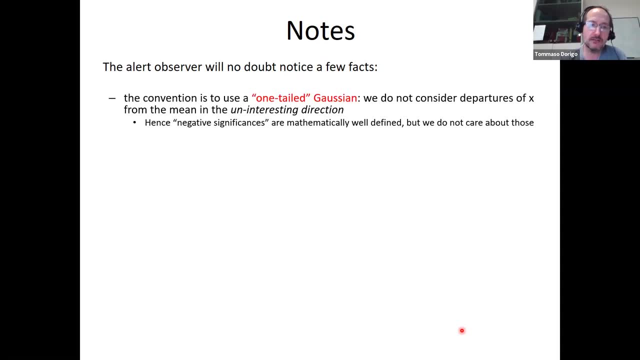 events. so we look in only one direction, Not always, but typically, Typically yes, And the conversion, of course, is just a mathematical map which allows us to talk more freely about the small numbers Of course we have to. 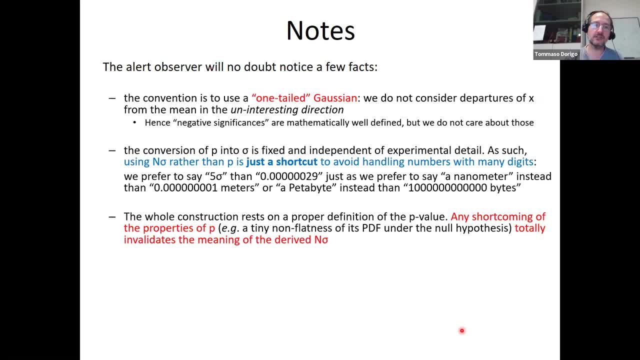 compute p-values correctly and otherwise our number of sigmas will be meaningless Very quickly we become meaningless because very small p-values are very hard to estimate correctly And I will show how the tails of our systematics are known Gaussian later on in the talk. 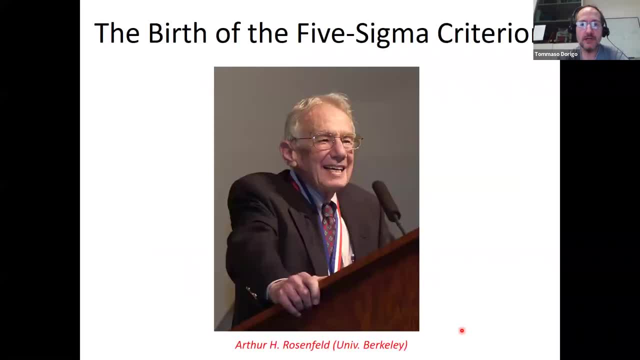 Okay. so this is a very small p-value which is very hard to estimate correctly, And I will show how the tails of our systematics are known Gaussian later on in the talk. So I'm a little bit behind with time, so I will briefly talk about the birth of the 5 sigma criterion. This is a physicist at Berkeley that realized in 1968 that physicists were looking for new particles by looking in many boxes. 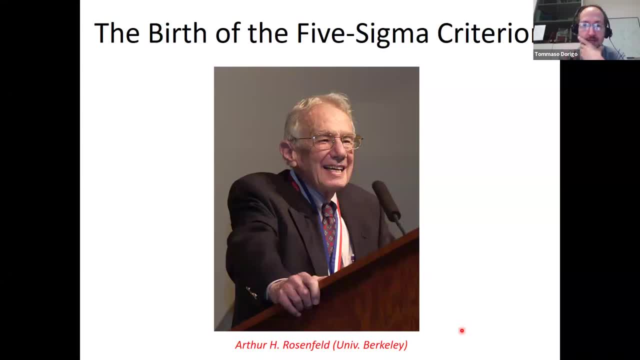 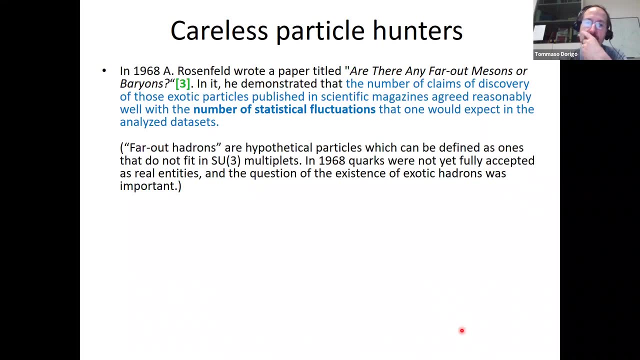 So I will briefly talk about the birth of the 5 sigma criterion. This is a physicist at Berkeley that realized in 1968 that physicists were looking for new particles by looking in many boxes. Okay, let's put it this way: They were looking for many, many histograms, and the problem was that there could be exotic particles that were not made of three quarks, or quark and quark. Okay, let's put it this way: They were looking for many, many histograms, and the problem was that there could be exotic particles that were not made of three quark. Okay, let's put it this way: They were looking for many, many histograms, and the problem was that there could be exotic particles that were not made of three quark. 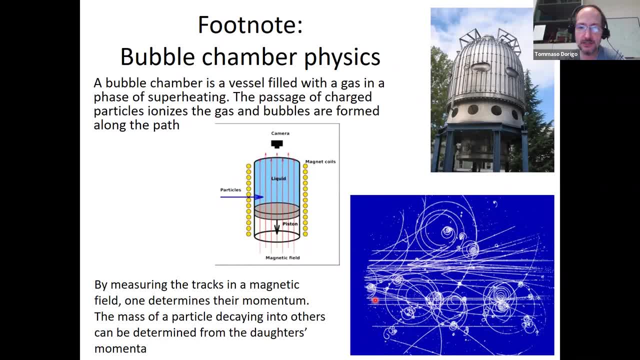 Okay, let's put it this way: They were looking for many, many histograms, and the problem was that there could be exotic particles that were not made of three quark kind of detectors that are called bubble chambers, but I won't describe what they are, but you. 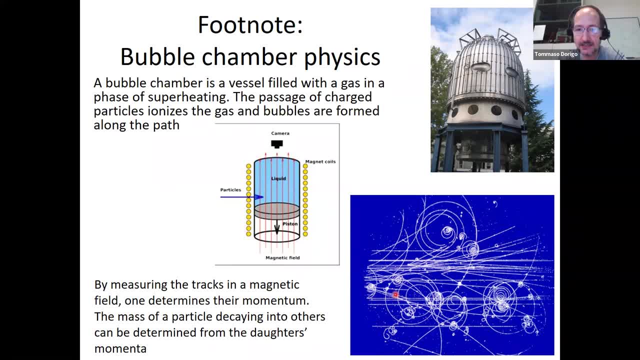 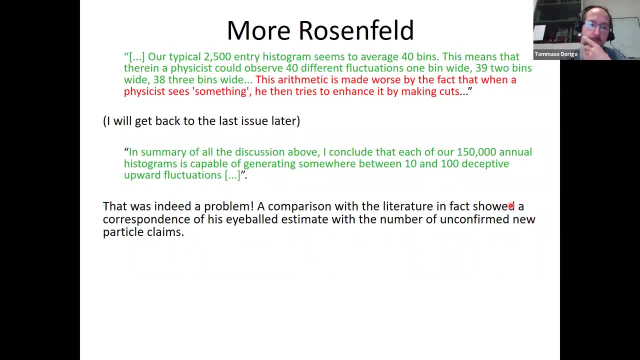 can see that the particles leave track in a gas and then they can be tracked and you can compute mass of particle pairs or triplets and then produce histograms. So he pictured the situation, which required some mending. And so he said to the theorist of phenomenology: the moral is simple. 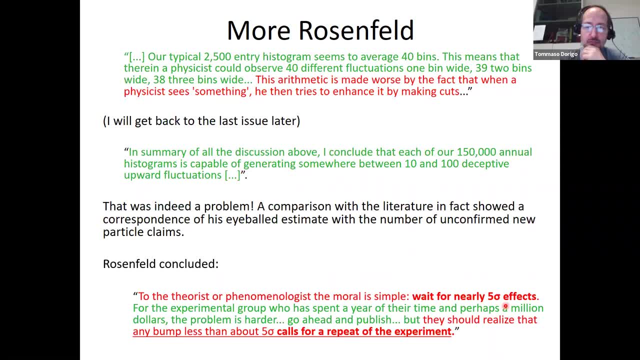 Wait for nearly five sigma effects because he estimated that this would cut all of these spurious effects. But for the experimental group, who have spent a year of their time and perhaps a million dollars, the problem is harder. You want to publish, but they should realize that any bump less than about five sigma calls 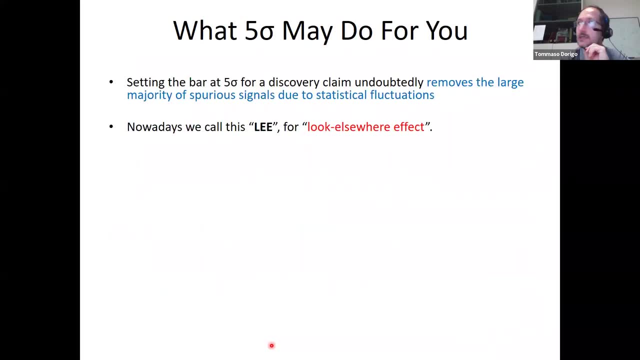 for a repeat of the experiment. So what five sigma does for you is that reduces these spurious claims. In physics we call this look elsewhere effect. That is, we have a multiplicity of possible searches because we have a nuisance parameter. So the mass, for instance, is not defined. 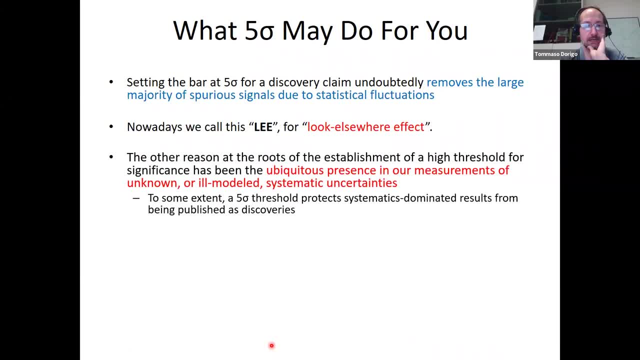 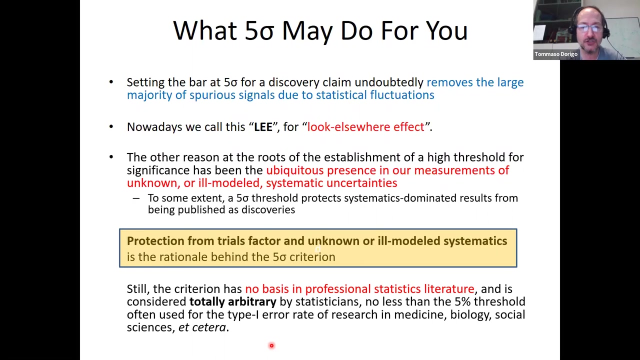 So we look in many, many possible mass values, And then of course there are ill-modeled or known Gaussian systematic uncertainties that can sort of mess up our estimation of the significance. And so protection from trials factors And unknown or ill-modeled systematics was the rationale behind the five sigma criteria. 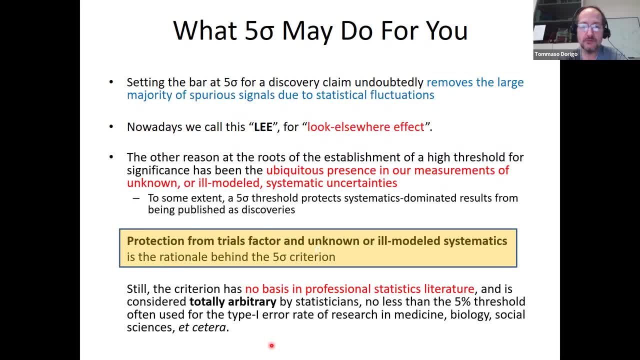 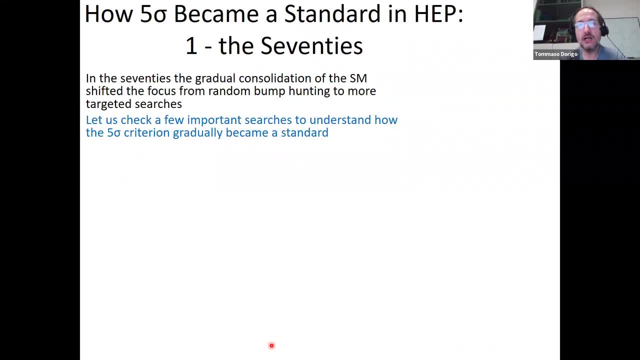 You know better than me that this criteria has no basis in professional statistics literature, no more than the 5% that is used in medicine. Very quickly, because I have little time, I will just walk you through the most important discoveries that were made in high energy physics. 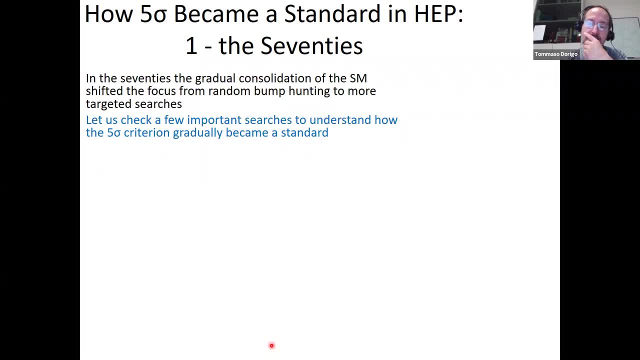 That This slowly coalesced with this idea that we should wait for large effects. But it took a while because in 1974, quarks were discovered. by finding this particle called the Jape side caused the five Nobel Prizes, And this is the peak that was seen. 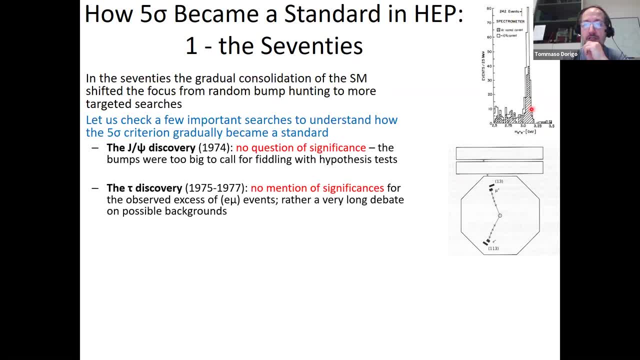 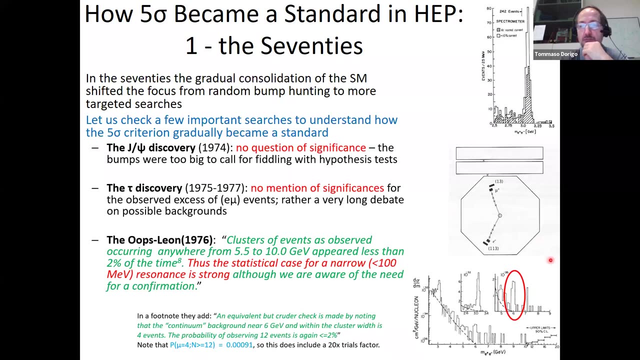 You see, there is no question of significance when you see such a towering effect. And the tau lepton was also not a question of statistics analysis Whether these funny events found at Slack were a new lepton or not. And then a spurious signal was observed when looking for a causing of this particle made. 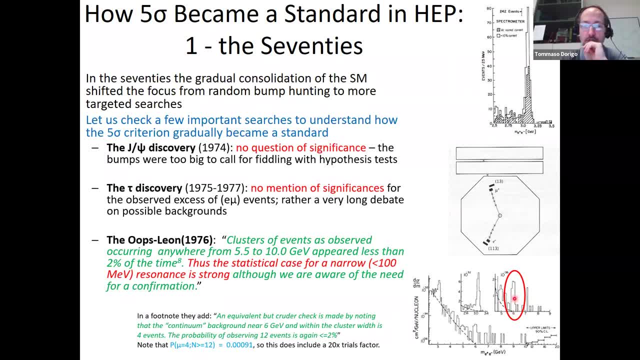 by a heavy quark called the bottom quark that was later discovered by the same experiment. But here they published this effect and it was due to their multiple testing in a wide range of histograms. Uh, And they did account for a trials factor in their estimate. but they published something. 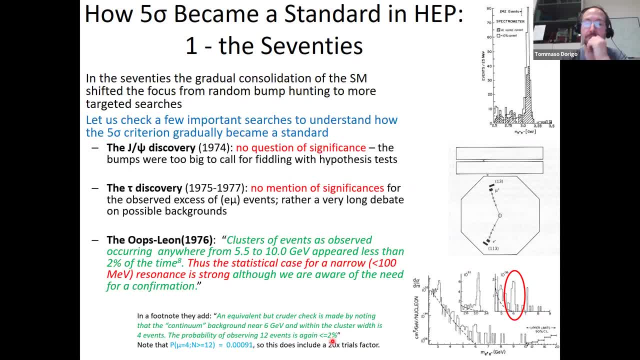 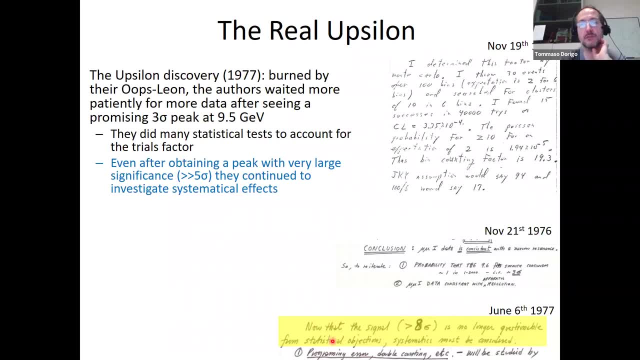 which could have an error rate of 2%, So it was not a very significant effect. They published it and then they retracted it and they studied the matter much, much, much in more detail And when they eventually found the particle, this is a background subtracted plot where 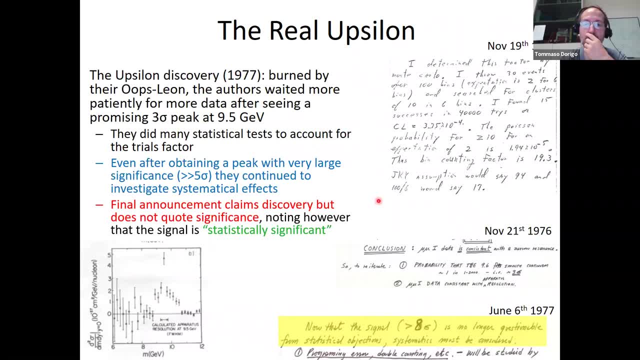 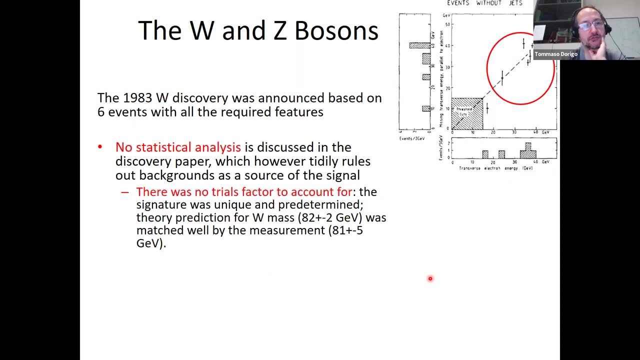 you see a very towering peak. They waited a lot before actually getting to publish. So This is a failed application of the five sigma criterion that was still in the making. And also when Rubia discovered W and Z bosons at CERN in 1983, there was no statistical 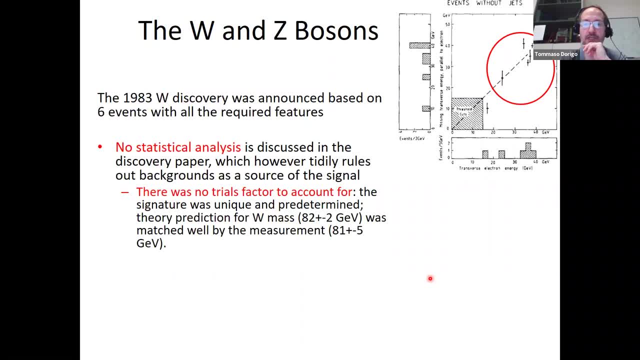 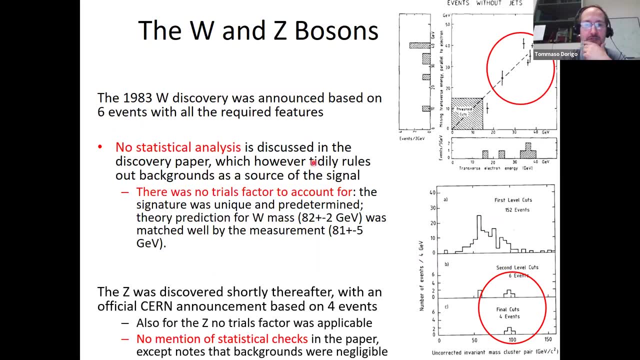 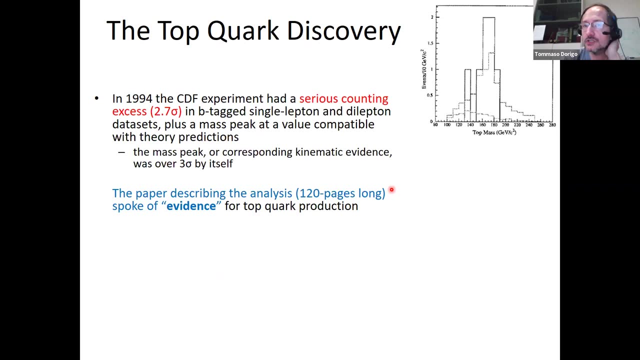 analysis, It was just proving that there were these funny events that could have no, no way to arise out other than if these particles were the cause. So we, really we, had to wait 1994 for a duty duly application. Uh, 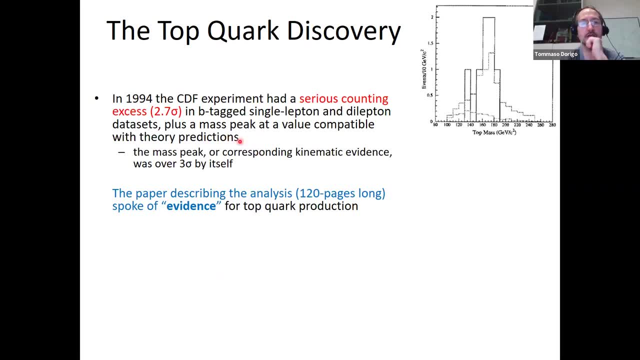 This is an interesting application of the five sigma requirement because the experiment that was in CDF found a signal of top quark. This is the reconstructed mass of the top quark found in 1994 by CDF, where backgrounds would have accounted for only this small histogram here. 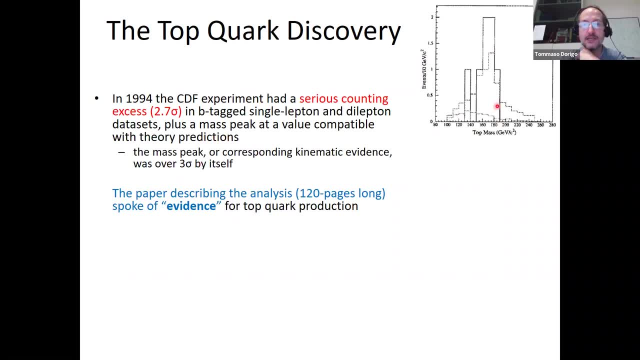 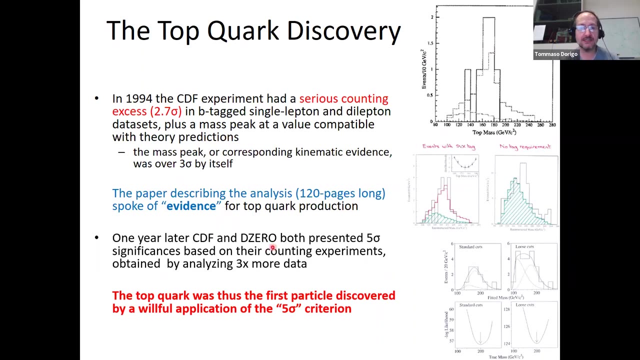 They had a count in excess of three sigma but they also had a systematic effect on in the mass distribution. But they decided to call it evidence for top quark production And so production in their paper. So one year later, more data collected. There was another experiment. 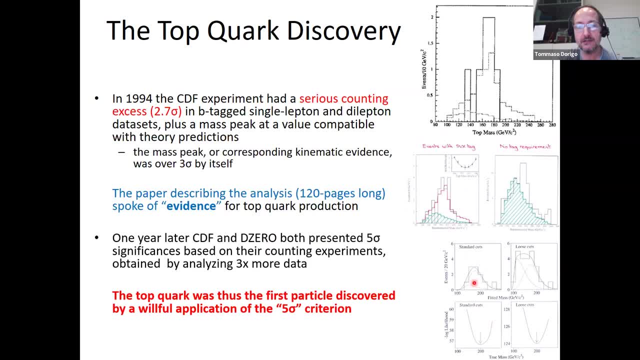 across the ring and the two experiments together discovered the particle by finding 5-sigma effects. But this cost CDF, the actual patronymity of the discovery. So this was the first particle discovered with a willful application of the 5-sigma criterion. So we call 3-sigma an. 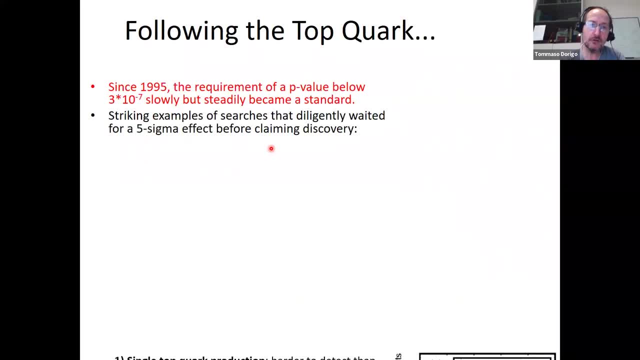 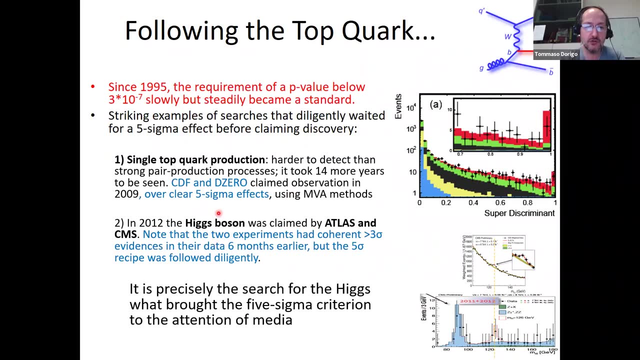 evidence but not a discovery, And following the top quark, there have been other examples. I won't go through them, but of course, in 2012,, this was the X-Boson discovery that brought this 5-sigma criterion to the. 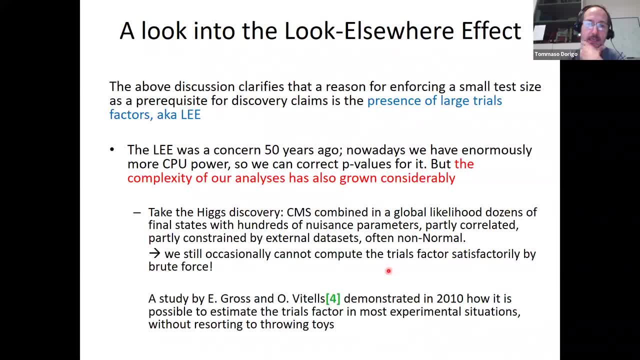 headlines of the press because it was widely distributed. So a reason for enforcing the small test size- 10 to the minus 7, is the presence of this large trials factor. It was a concern 50 years ago, but now we have computing that allows us to actually. 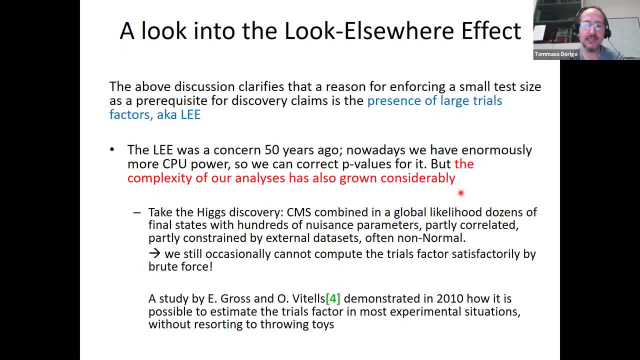 measure the trial factor. But still sometimes it's hard to do because in the X-discovery, for instance, we combined in a global likelihood dozens of final states, hundreds of nuisance parameters, funny PDFs, so it's not easy to compute the trials factor there. There is a study that 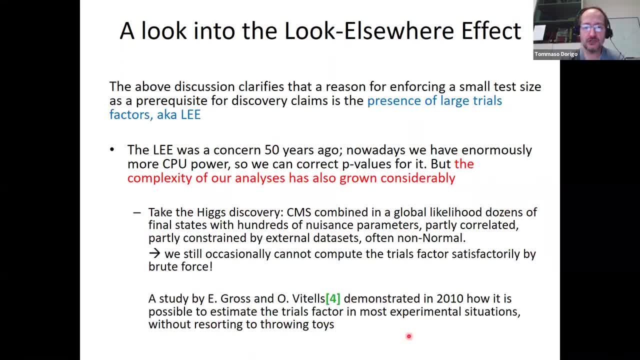 is done by physicists- my friend Deyla McGrath. They demonstrated how to account for the trials factor in a precise way in the business that we do. Now I don't have the time to go through it very quickly, although if we ask for a question later I can describe it. 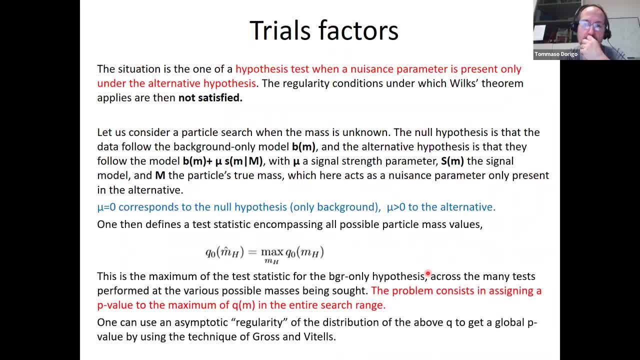 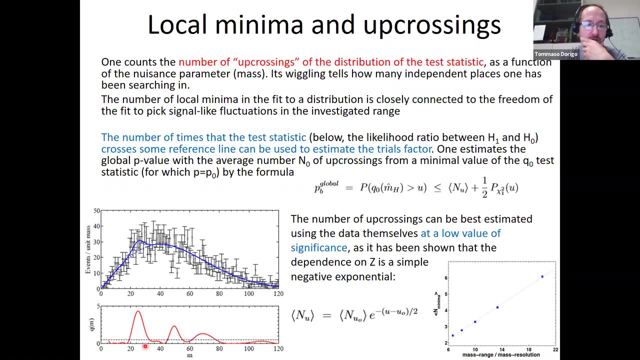 The method is, very quickly, very simply put, based on constructing a maximum of test statistic over the unit time limit- Okay, nuisance parameter- and then looking at how this test statistic wiggles around as a function of the nuisance parameter, because how often it wiggles up and down a certain threshold. 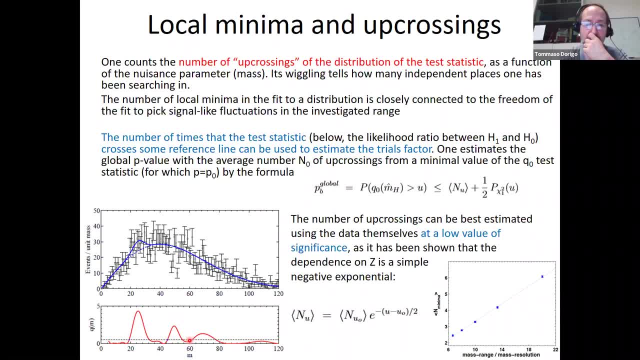 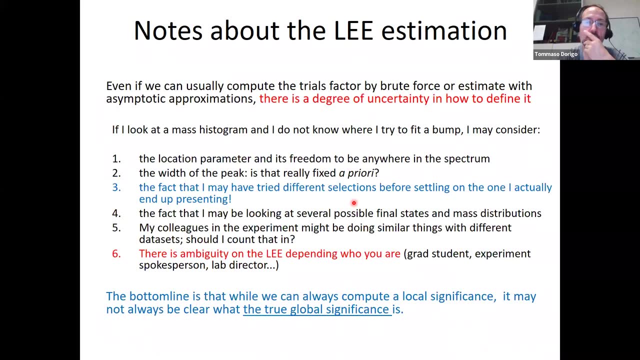 tells you how many different searches you are effectively making. And then there are formulas that allow you to get the global p-value from the local one. Sorry for being very quick on this, but if you are interested I can be more exhaustive. So even if we can compute this correction and then get a global significance, it's kind. 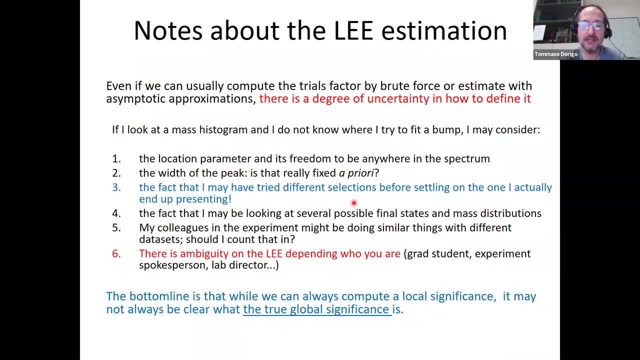 of silly to do, because it's very well, very ill-defined. You can, of course, consider the location of this nuisance parameter to define how many boxes you have looked into effectively. But then you might ask: well, but you have looked for particles of a certain PDF, so 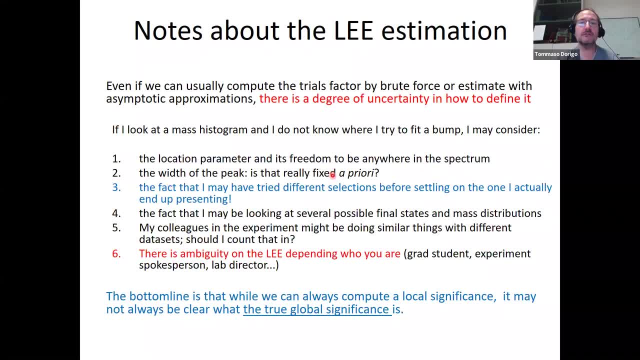 with a certain width, Is that of the Argosian peak, And is that really fixed? No, it's not fixed. So you should take that into account And this actually has been done in another paper by Gross and Vittels, but it's beside. 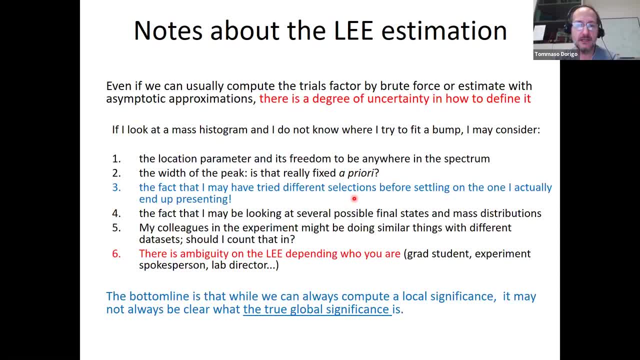 the point. The point is that there is an ill-definition of this quantity, the trials factor. You could have tried different selection cuts to put in evidence the signal, and this actually is done by physicists. So And also you could have collusion. 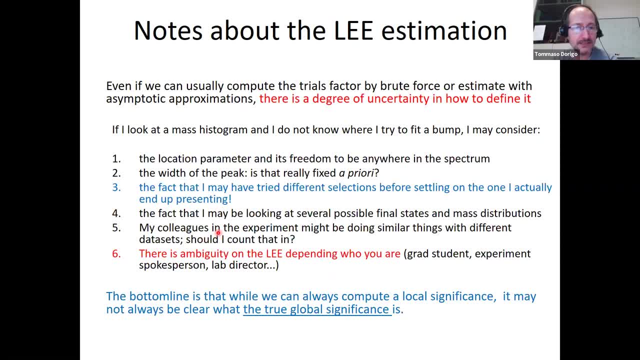 You could have colleagues that search for the same particle in different ways. So when somebody goes up to the spokespersons and said: look what a signal I have found is just one in 3,000 people and you should account for that too. 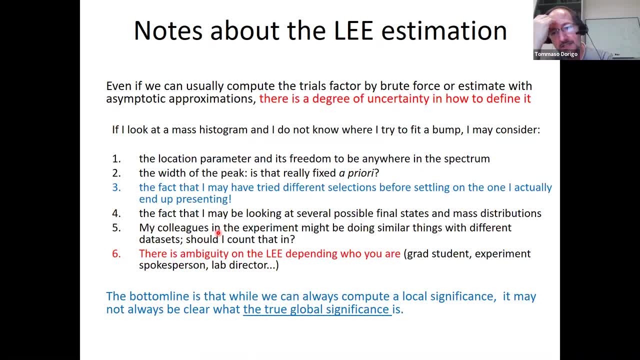 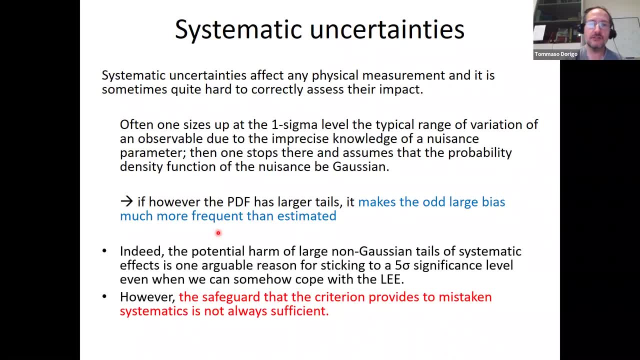 So the bottom line is that while we can always compute the local significance, it's not always clear what the true global significance is. And then there are systematic uncertainties that affect any physical measurement. So typically we don't know how to estimate. And you can try to size them up at the one signal level, but then when you are extrapolating, 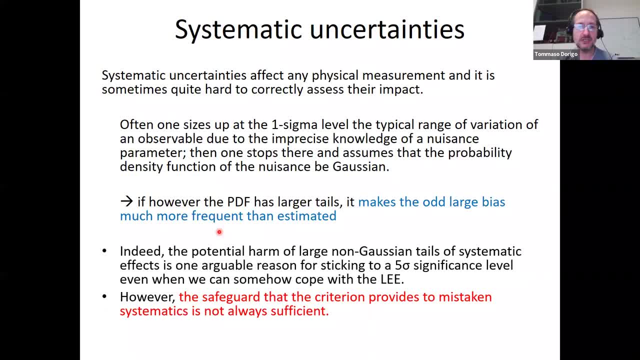 to five sigma, you are liable to get very bad mistakes right, Because if the PDF is not Gaussian then you are in trouble. So, indeed, the potential harm of large non-Gaussian tails is argued to be why we stick to five sigma requirements, even when we do not have such a large trials factor as it was the case. 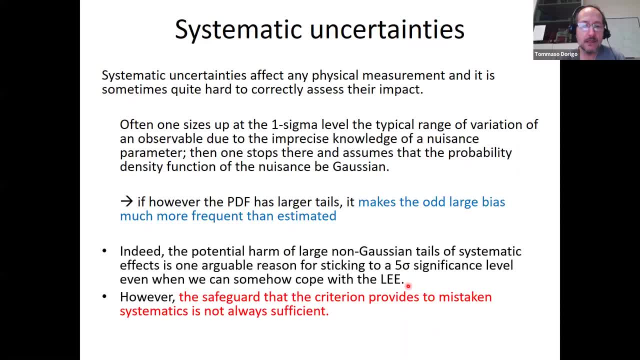 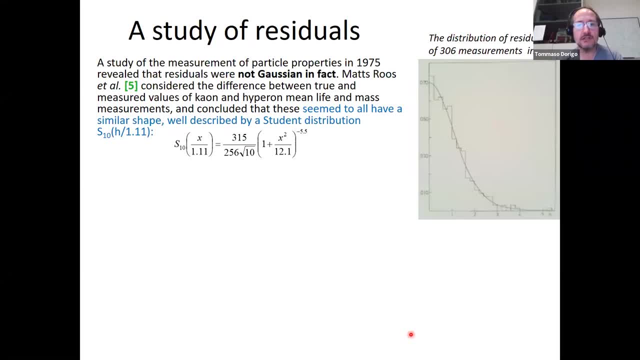 for the data, The single top discovery, for instance. So in any case five sigma may not be enough in some cases. There was a study of residuals in 1975 using particle physics measurements of particle physics properties done in particle physics experiment by particle physicists. 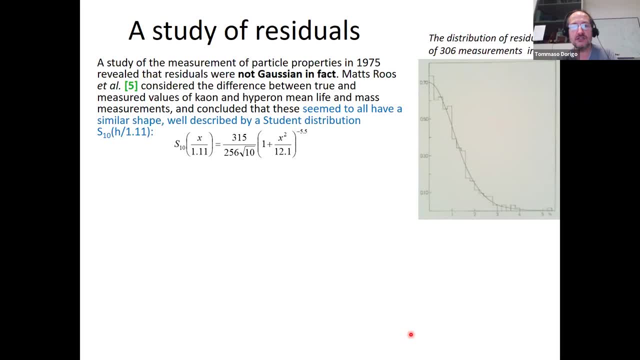 This guy proved that particle physicists do not estimate their systematics well enough because it could get a residual plot like the one you see, which is not Gaussian but the student distributed And you know a student distribution has longer tails and in fact, if you compare to a Gaussian, 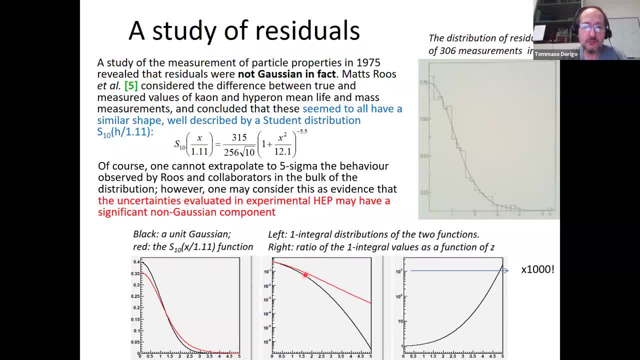 by the time you hit five sigma, the ratio between such a distribution and a Gaussian is a factor of 1,000. So this tells us that we should be very, very careful. okay, Because this is published measurements and we wear off in estimating our systematics. 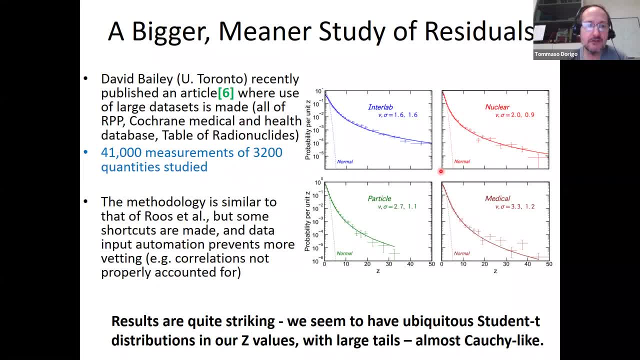 There is even a bigger, meaner study of residuals done by David Bailey, Which showed that this is a pathology which is common to many different areas of research, Where you see that the Z values, the significance for a normal distribution, would give you residuals. 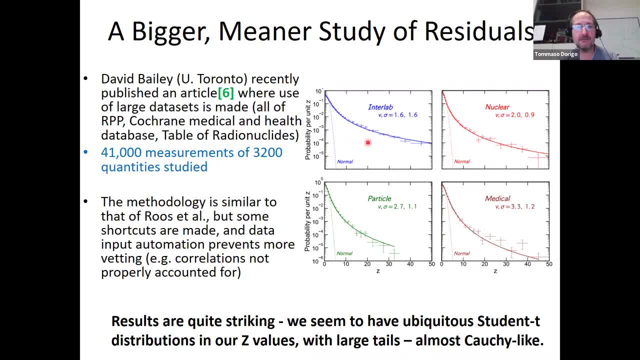 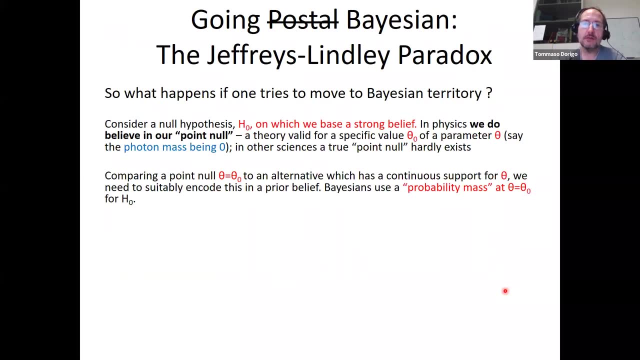 in this range, while they extend to very, very higher values. okay, So we should be very careful with our systematic uncertainties, or nuisance parameters, as you call them. Can we solve these problems by going Bayesian, not postal? So there is one paradox, called the Jeffries-Lindley paradox, that forces us to take a pause before. 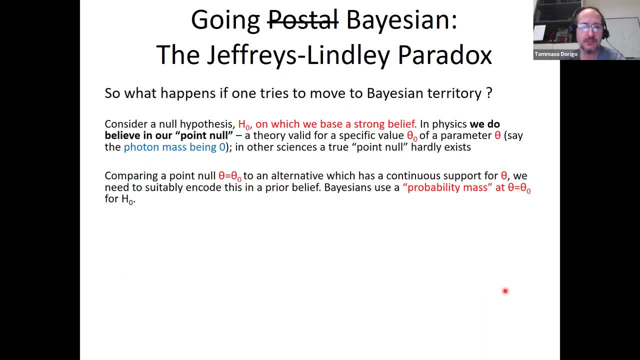 we start using Bayes factors for this business, Because typically we have a null hypothesis, say the standard model on which we base a strong belief. And this is a point. null distribution- Okay, It's not a distribution in your jargon, right? 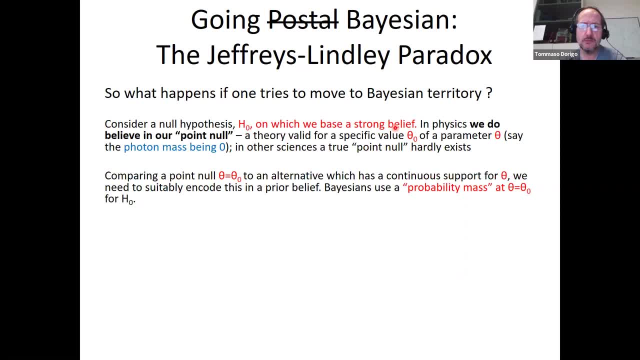 It's something that is valid for a specific value of a parameter. In other sciences it's hard to find point nulls, but for us it's very common. The photon mass is zero. The number of protons and electrons in the universe is the same stuff like that. 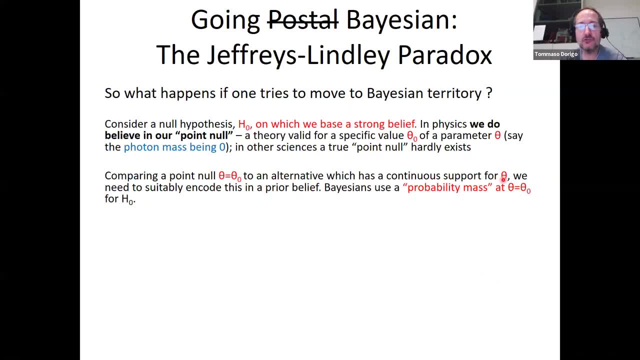 If we have to compare a point null to an alternative which has a continuous support for theta, so it is governed by the nuisance parameter. We need to encode this. We need to encode this in a prior belief in some way. So we will use a probability mass at theta equals theta zero for the null. 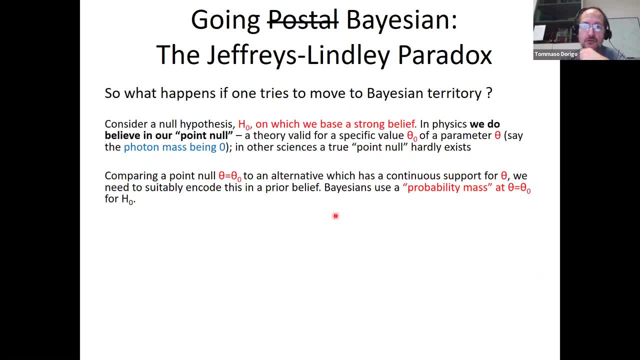 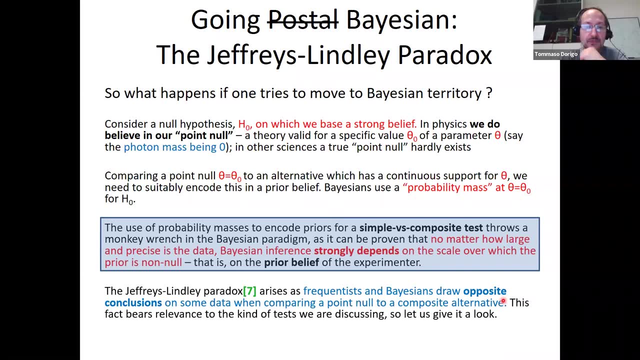 And then we will distribute the rest of the probability over a range of values for theta. Well, if we do that in a simple versus composite test, then we break the Bayesian paradigm, Because we can then prove that no matter how large is your evidence, that is the amount. 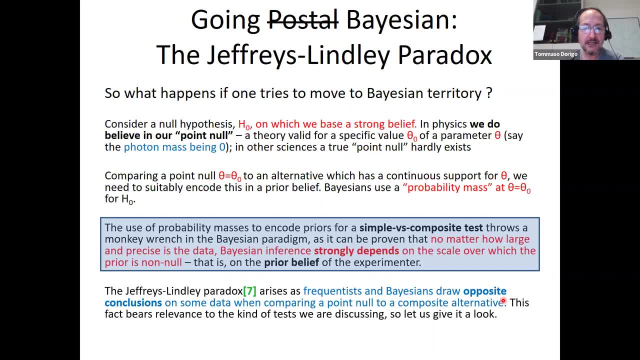 of data that you throw at the problem. Okay, The Bayesian inference that you will do strongly depends on the scale over which the prior is non-null, That is to say, the paradigm that the prior that you choose doesn't matter any longer when you have a strong evidence, when the data speaks loud, is not true. 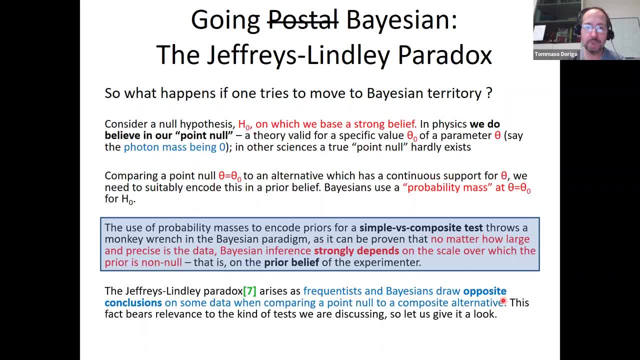 Because this singularity of the point null really breaks this. Okay, Indeed, the Jeffries-Lindley paradox is mentioned. It's mentioned as saying that frequentists and Bayesians will draw opposite conclusions on some data when comparing a point null to a composite alternative. 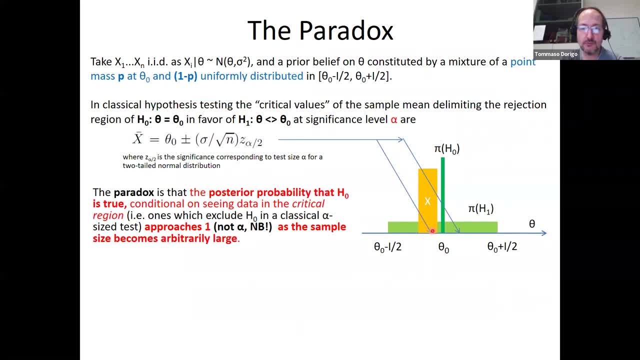 And this arises because, as your data becomes more precise, you have a certain scale for the uncertainty on the measurement and you have a scale for the prior, which is basically a Dirac's delta, and you have a scale for the alternative prior and so the existence. 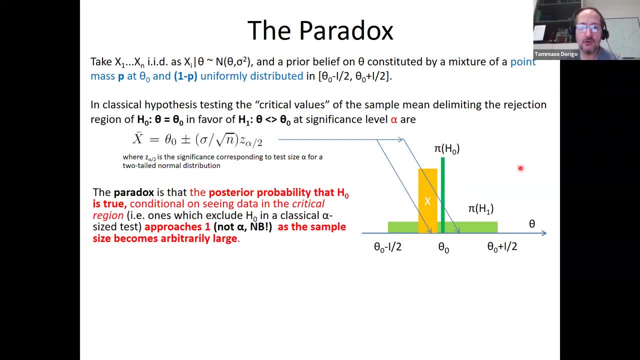 of these three scales In the problem is what causes Bayesians and frequentists to asymptotically reach opposite conclusions on this? The posterior probability that the null is true, conditional on seeing data in the critical region, that is, the one that would exclude the null, approaches certainty as the sample. 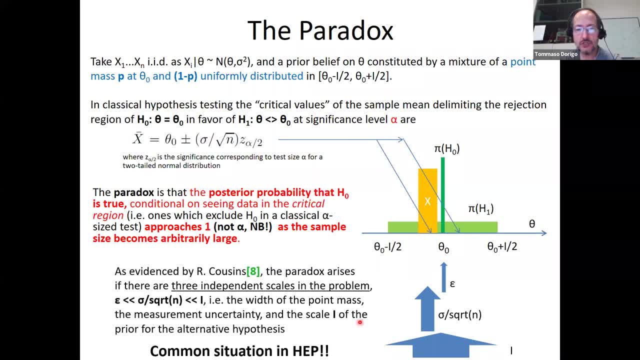 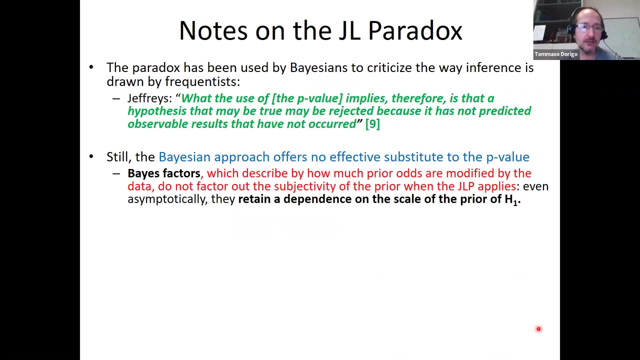 size becomes arbitrarily large, This is due to the existence of the null. This is due to the existence of these three scales in the problem, And this is a very, very common situation in high energy physics and that is why it's kind of hard to move to Bayes factors to decide on discovery level or evidence or stuff like. 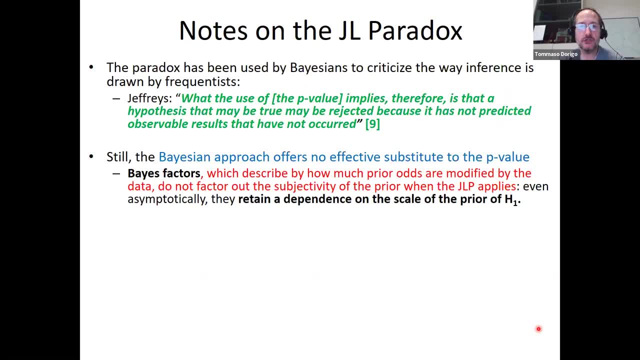 that. So this is an active area of research. The paradox has been used by Bayesians to criticize the way that inference is drawn by classical statisticians. So Jeffries-Lindley paradox, So Jeffries himself is quoted as saying what the use of the p-value implies is that 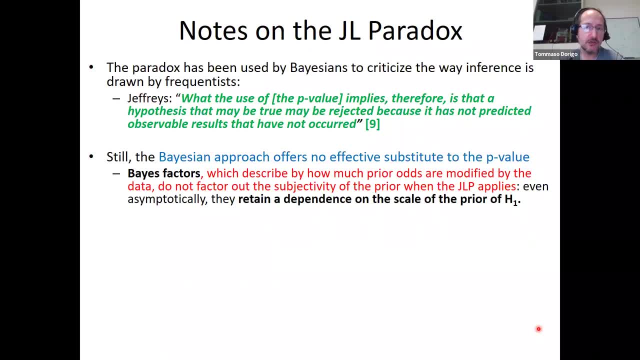 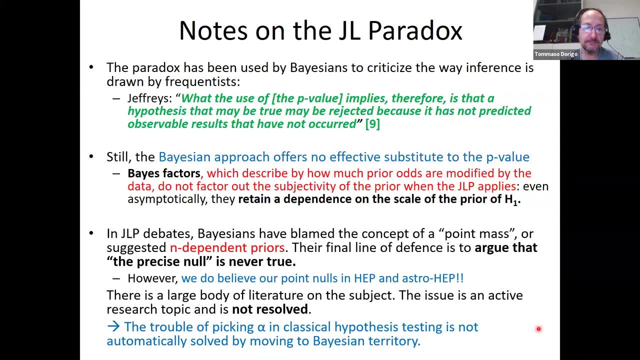 the hypothesis that may be true may be rejected because it has not predicted observable results that have not occurred. So this is a famous quote. But so Bayes factor will retain a dependence on the scale of the prior, on the alternative. There have been attempts to mend this by using the P-value. 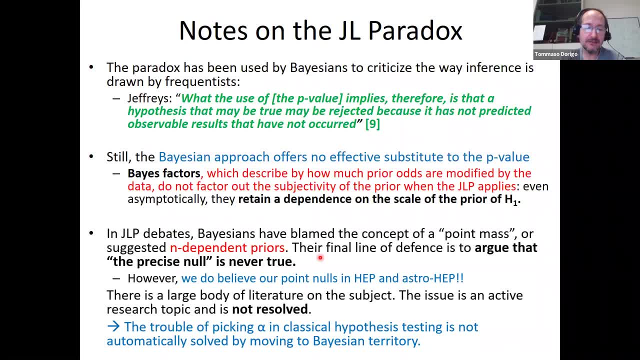 Okay, Evidence dependent priors. but or to argue that the precise null is never true. but in particle physics this is actually the case. So we will not resolve the issue today. but the trouble of picking the type one error rate in classical hypothesis testing is not automatically solved by moving to Bayesian. 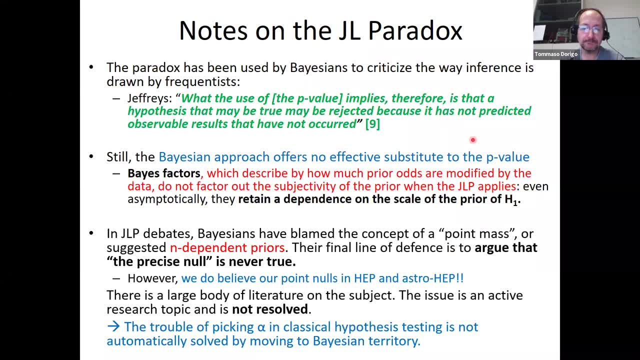 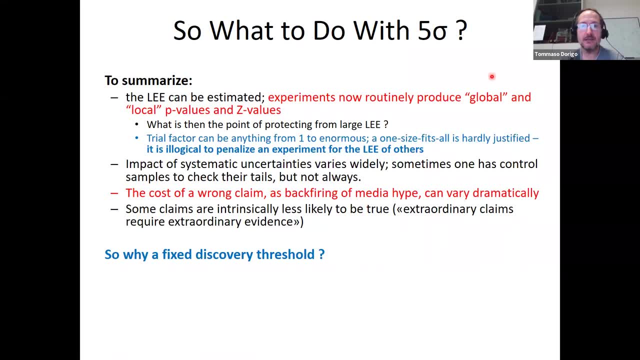 territory in the case of this kind of inference. So what should we do? Yeah, About five minutes, I'm done. I'm done, Yes, I'm actually done. So what we should do with Phi Sigma is that it's a good reference value, a useful standard. 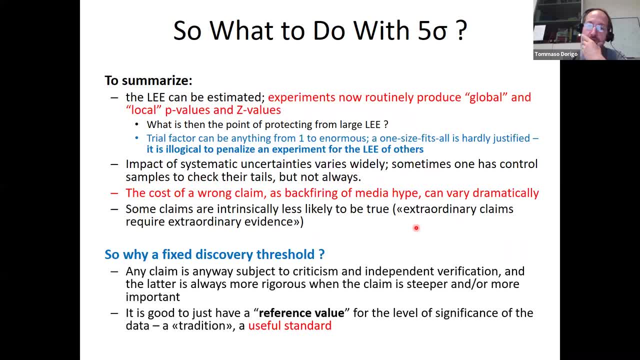 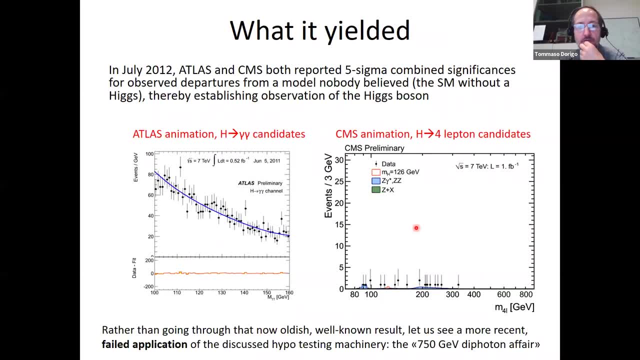 for our field, and it doesn't protect for false claims. I have just an example for this, and then I'll wrap up. So first of all, I let you see how the X boson data allowed us to draw inference on its existence. 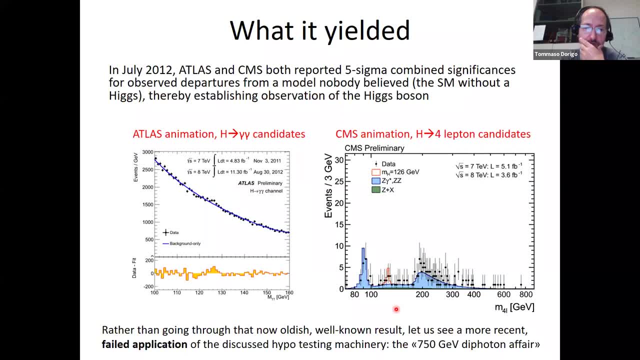 So let me just show you this by collecting the data, Just because these GIFs are too good not to show them. you see that in two different channels of X decay, the two experiments found this narrow, these small peaks, as they collected more data. 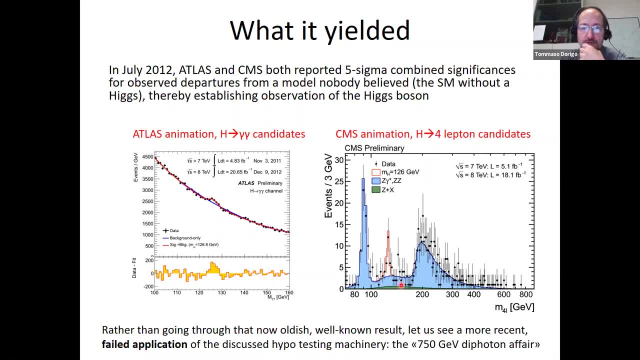 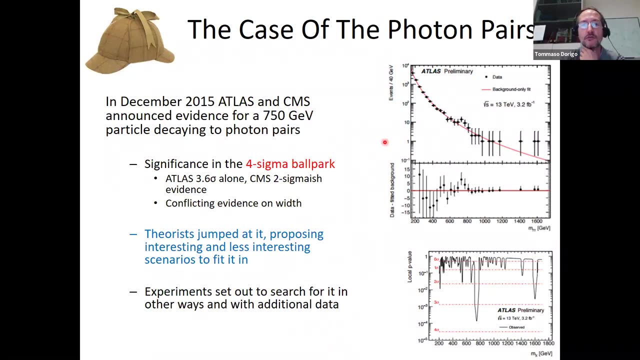 So this was a successful application of the Phi Sigma criterion because indeed later on we even got stronger evidence. so this is a real particle. Okay, So it was five years ago a claim that the two experiments put forth still in the diphoton. 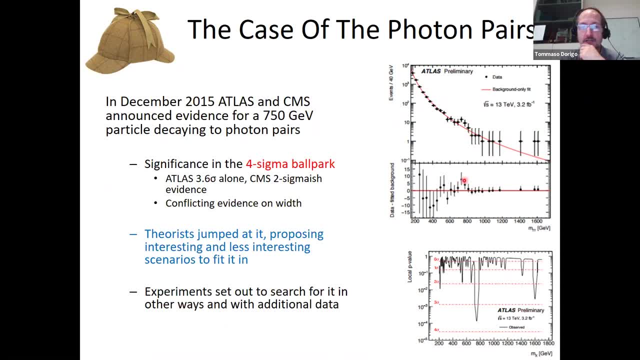 final state that there was a particle that had a mass of 750 GeV, that behaved like a X boson, and they based this on this histogram and a similar one by CMS, And this created havoc because theorists jumped at this possible new signal proposing 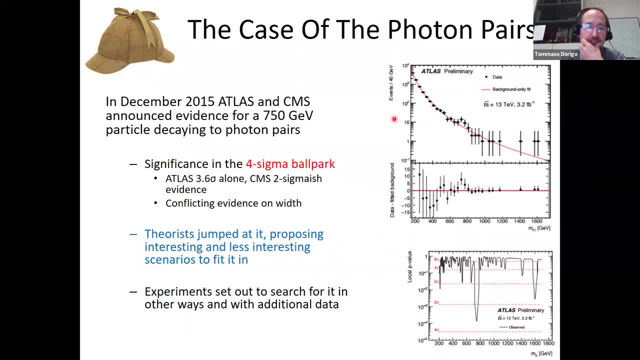 a number of techniques. So this is an example of theories that could allocate such new particles. Experiments tried to find more evidence. this, you see, is the local p-value as a function of the mass for this histogram and you see this as almost four sigma effect, but it was. 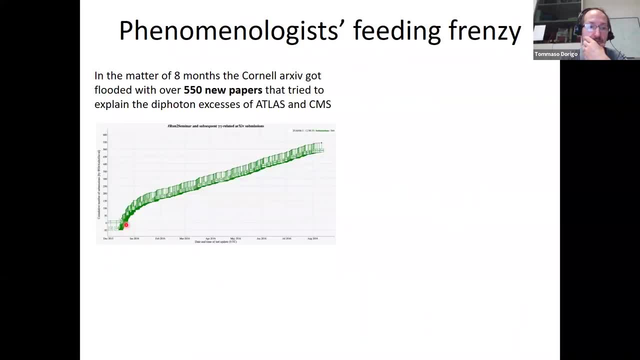 not confirmed with more data. In the meantime, though, theorists published. you see, as a function of time, they published almost 600 papers. I think in the end, the number is almost close to a thousand papers, Because this graph has continued to grow. 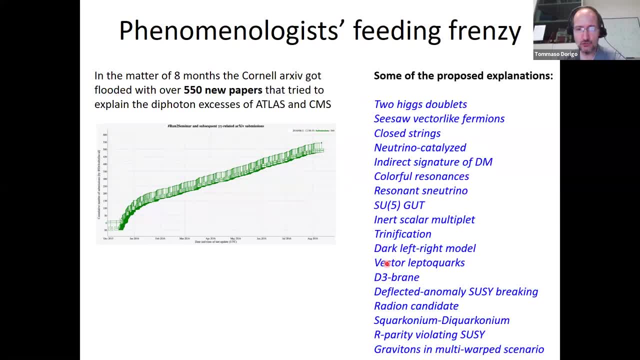 So the point is that they put forth a huge number of possible explanations for a phenomenon that was not confirmed Because it had not reached five sigma. but even if it had, I would argue that this is kind of an insane way of doing our business, right, because you have thousands of theorists. 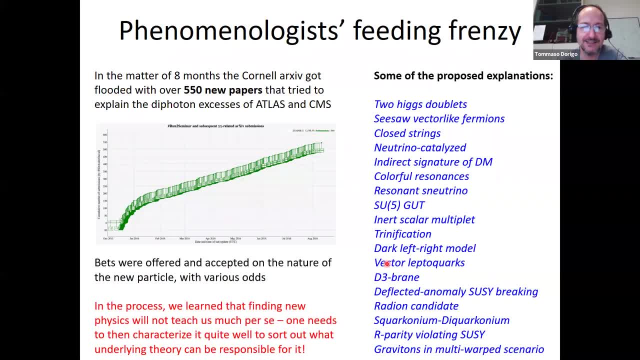 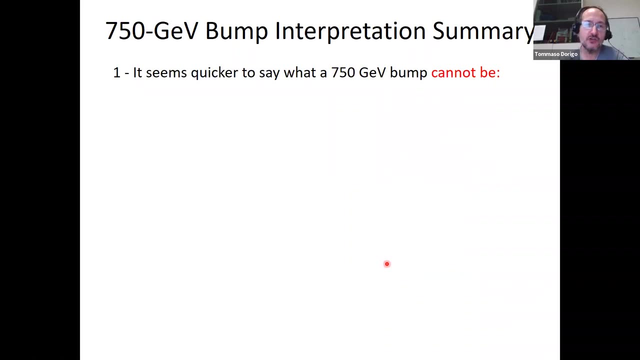 that thought for one year, over Christmas and everything, to find an explanation for something which was not real. So in the process, we also learned some good physics. What we could say after having examined all these models is that so this is a joke, but 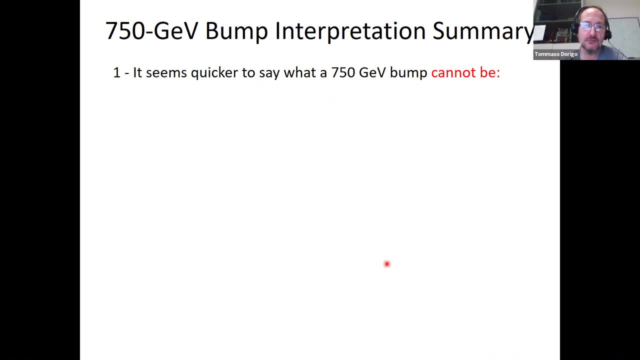 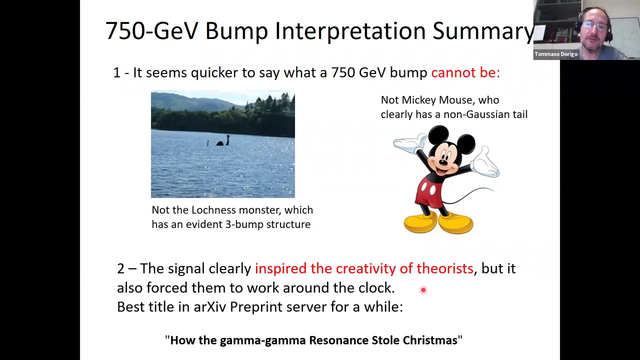 it was. I argued in a conference that it seemed quicker to say what the particle could not be. And it could not be the Loch Ness Monster because it had a three-bump structure And it cannot be Mickey Mouse because it had a non-Gaussian tail. 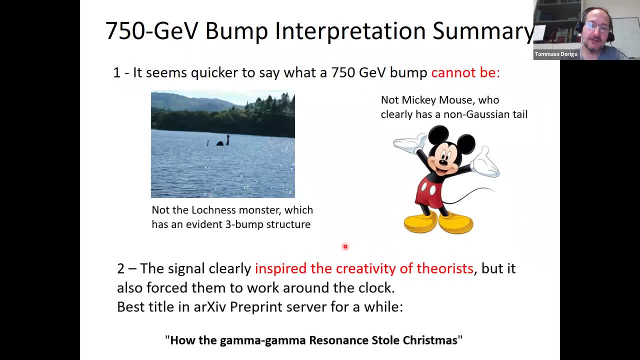 So And- And it is a joking matter- because of so much effort on the bright minds on nothing really. So the best title in the archive for print server for a while was how the gamma-gamma resonance stole Christmas, Because really these guys were working over Christmas to try and explain this phenomenon. 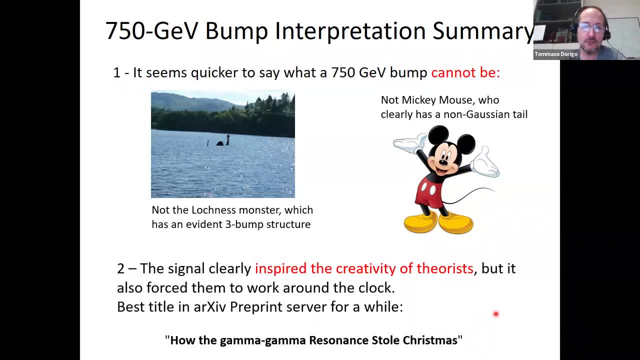 which was spurious in the end. But what it teaches us is really we need the prescription and but it's not even. it's not enough, Because even if the prescription is followed, because Atlas and CMS did not publish a discovery of a particle, already the showing publicly of a graph that could hint at the existence, 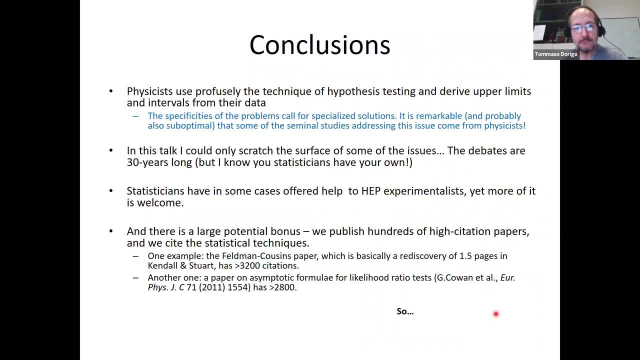 of something was a problem. So, in conclusion, physicists use profusely the technique of hypothesis testing and derive upper limits and intervals from their data, and their problems are quite special. I would say, And And some some look by statisticians over the shoulders of physicists, behind the shoulders. 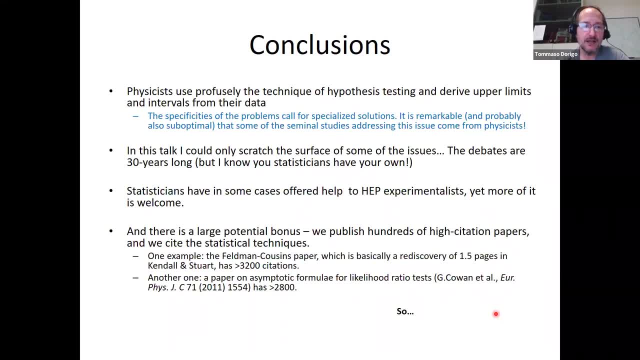 of physicists is advisable, I think- And this has been happening in fact, There are many debates surrounding these techniques- For statisticians to work in high energy physics problem carries with it a large potential bonus, because we publish hundreds of high citation papers. So to give you a couple of examples, 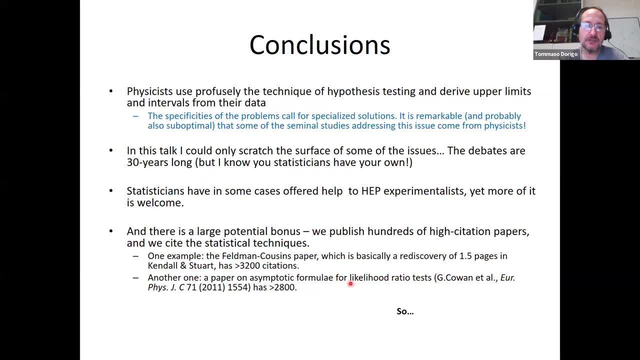 Okay. So to give you a couple of examples, there are two papers that that describe this. for instance, the Felman Cousins paper that describes this way of deriving upper limits, which is unified and solves the flip flopping problem, is basically a rediscovery of 1.5 pages in 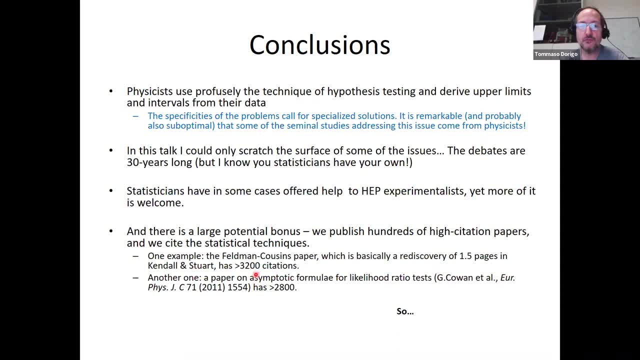 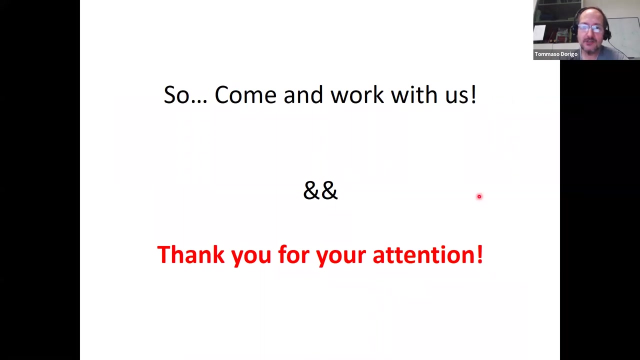 Kendall and Stewart, And it has acquired the 3200 citation to this day, And then another paper which creates a synthetic formulae for likelihood ratio tests which are used in our techniques. as collected, 2800.. So my message maybe is this: come and work with us, because it's fun and and there's 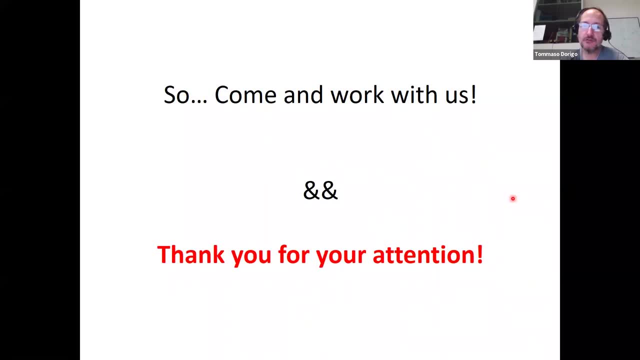 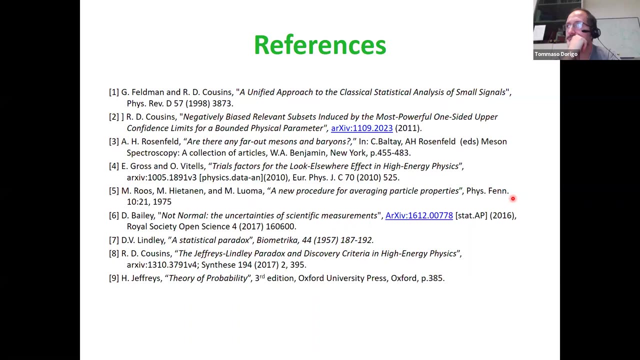 there's a possibility to break new ground. So thanks for your attention. Okay, Thank you very much, Tommaso. I am going to see a few hands raised here. I think Larry was probably the first. So, Larry, Can you go ahead and ask your question. 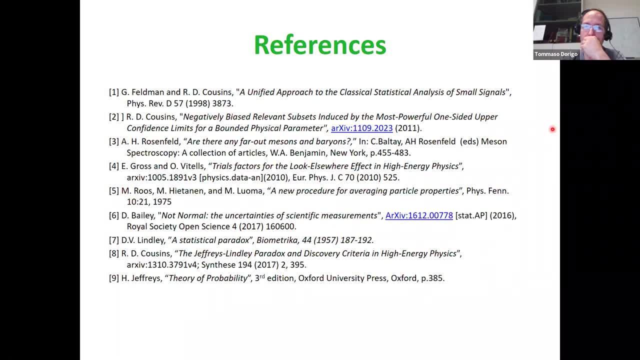 Sure, First of all, thanks. That was a very fun talk and I know it's dinnertime there, So I'm just. I was just thinking about the experiment some years ago where these people claim to turned out falsely that to discover that neutrinos could travel faster than the 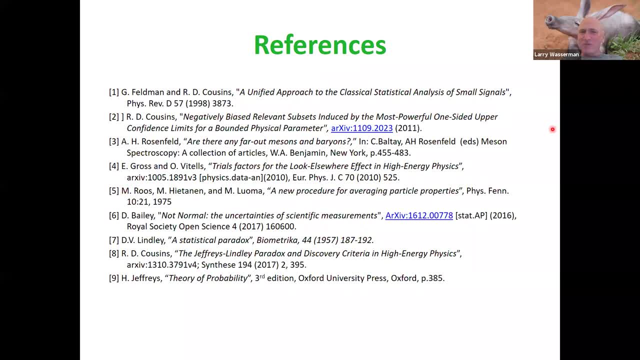 speed of light, And I was just wondering if you would comment on that and whether I don't remember now. Did they reach the five Sigma threshold? Yeah, It was a six Sigma effect because they had measured the timing of arrival of neutrinos. 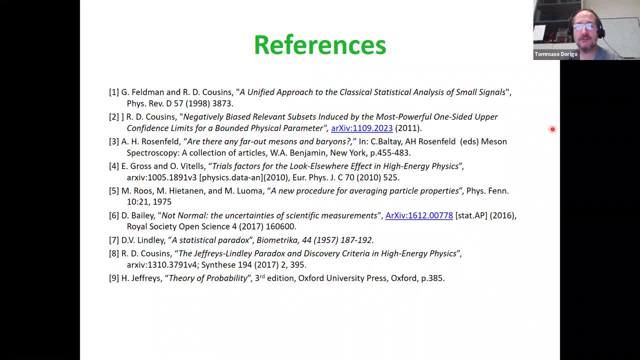 a bunch of them, 20 neutrinos, And it was a six Sigma away from zero, which was the time of a photon, say, because the neutrinos travel at the speed of light and not more. So yeah, this was in my talk, actually as one of the failed applications. 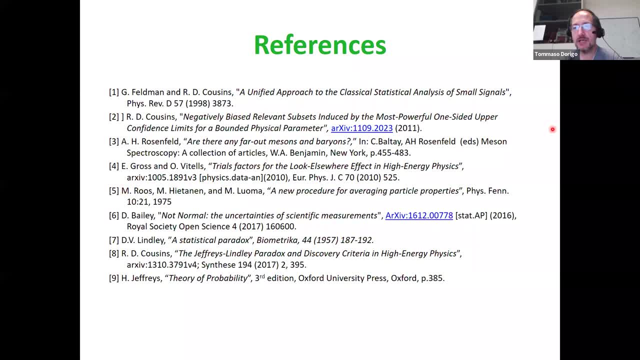 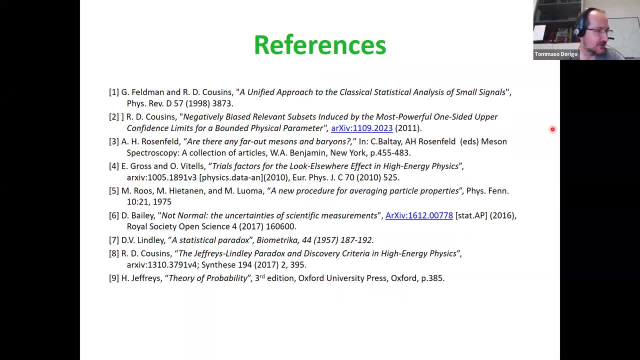 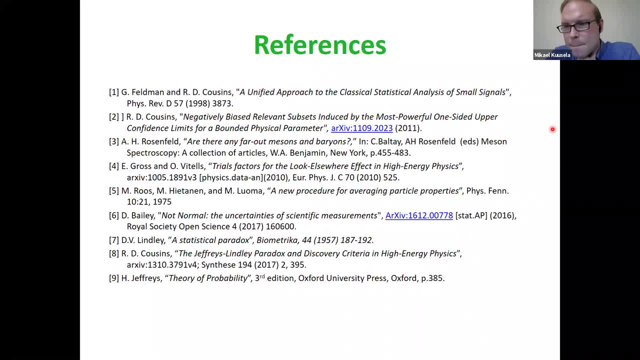 good example. They duly apply the distance. They said we have measured the best of our possibilities, this parameter that we say we don't find any mistake and the systematics are under control, and blah, blah, blah. And this is six Sigma. 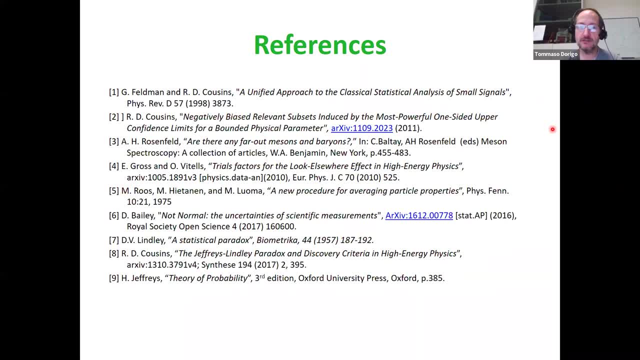 And people didn't believe it. I mean, the physicists didn't believe it because it's just too complex, steep of a claim to be believed, even at 310 to minus seven or less, right, I mean, it would really shake all that we know about particle physics to the roots. So what happened? 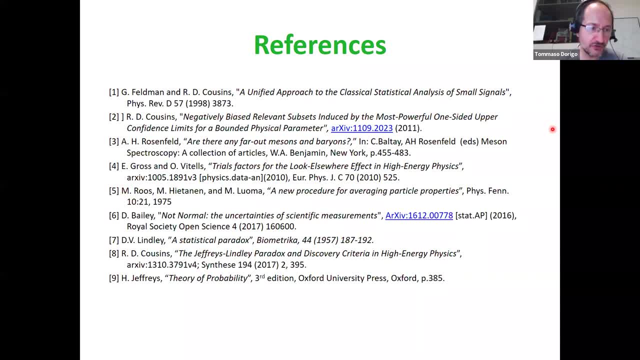 was that there were reanalyses, for checks, for data takings, and in the end, a systematic cause was found, which was just a loose cable, which reflected the signal and caused the delay of 60 nanoseconds. 60 nanoseconds is a very small time, right, But this tells you how hard are these? 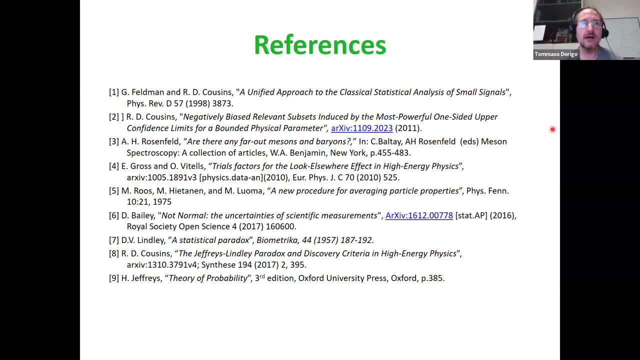 measurements and how careful we must be when we use our data to make steep claims. So, indeed, this is an example that, no matter how many sigma you are asking, there is a degree of belief that you have to. subject, There is a subjective belief that you have to fight when you want to convince somebody of 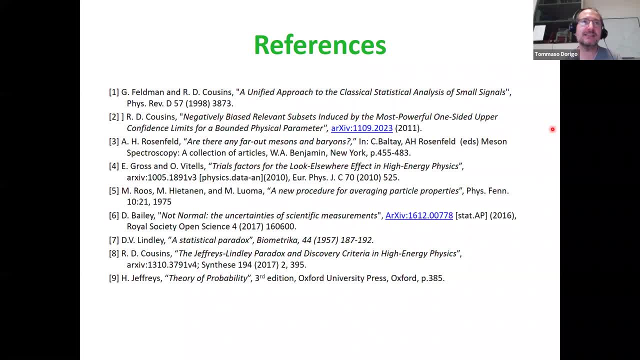 something. So this actually calls for some Bayesian flavor of doing this business, But that's just what it is. A fixed threshold will not protect. Thank you, Yep. Okay, And I think Pietro was next. Pietro, please go ahead. 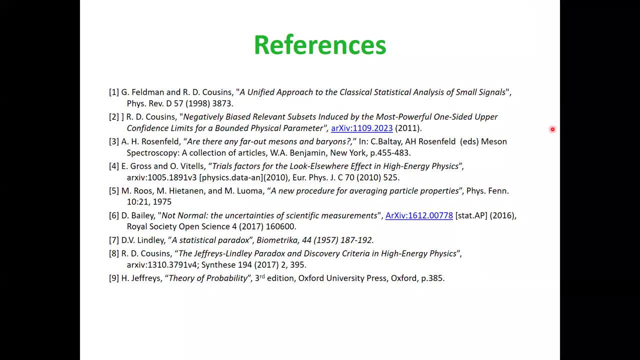 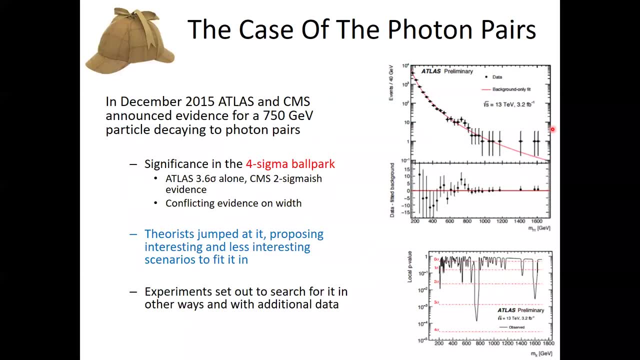 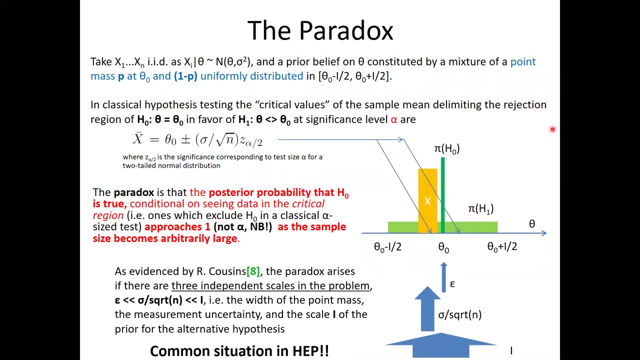 Yes. So concerning the difference, It's a paradox. So you rightly pointed out that one of the points is that essentially, for the point null, the measure is the delta, whereas for the alternative is a standard measure. So basically, in Bayesian statistics it's a problem having to treat improper priors And a few years. 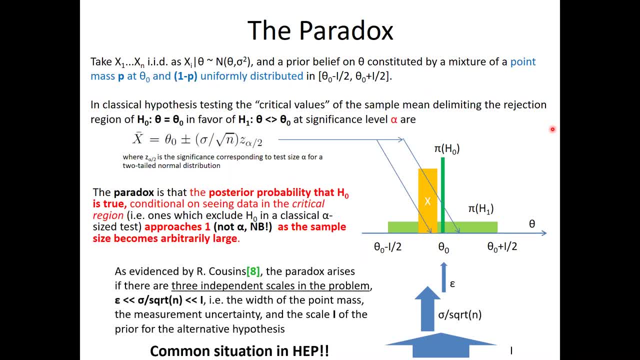 ago. I've come out with some ways of dealing with this that involve: Yeah, Instead of using the plane, the Bayes factor, you use some scoring rule that turn out to be independent from the normalization of the prior. Therefore, you basically remove the dependence on. 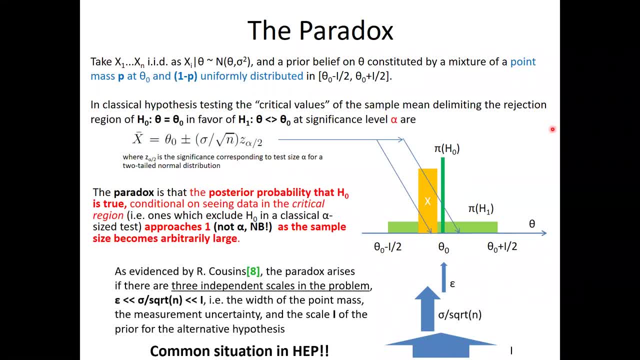 the number of events. However, they are usually not very light, at least in the literature we read, because they require to be calibrated. Yeah, Using an acceptance bound So, which is usually not very light in the Bayesian literature. But since it's something that we already, in particular physics, we already extensively do, maybe something that would agree with the taste of the physicist to have something that, I mean you have to choose an acceptance bound, but at least removes this kind of problems and might, you know, be able to do something with it. 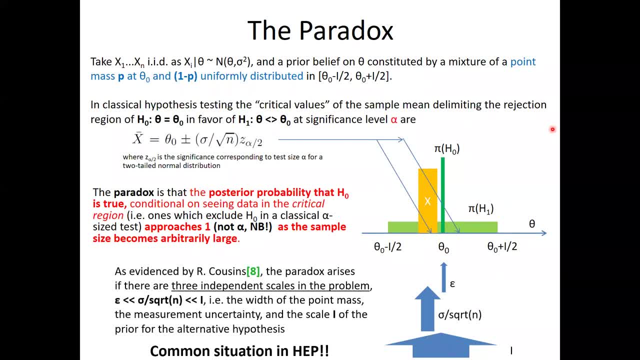 Yeah, I'm not aware of this. But the fact that I'm not aware of this- Sorry if I sound presumptuous now, But I mean, if something doesn't gain ground, it means that there is something in it that we don't like as a practice, or that makes it non-practical, or that there are other reasons to dislike it. I should look in the matter. But, as you say, in the end the field decides what to use and what not, also based on fashion, And so if this has not caused more interest in different ways of using Bayesian techniques, then I think it's a good question.